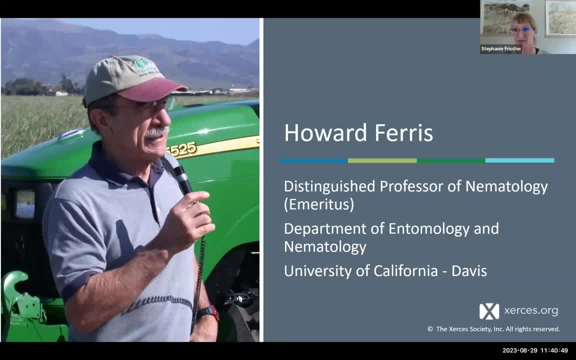 Our guest presenter, Howard Ferris. he is a distinguished professor of nematology, emeritus from the Department of Entomology and Nematology at the University of California Davis. Howard has conducted research on the biology and ecology of soil nematodes, both as pests and as 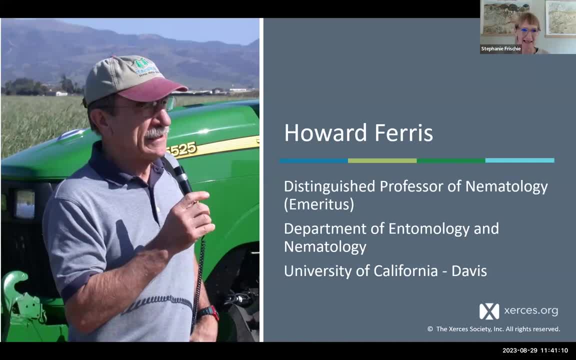 beneficial organisms, And he has this amazing website that he's going to be demonstrating called NemaPlex. It's an online resource of information on soil nematodes, their ecophysiological attributes and environmental impacts, including the host status of plants to the herbivorous nematode species. So with that I'll turn it over to you, Howard. 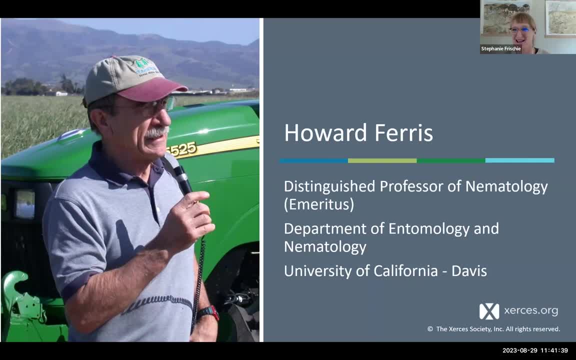 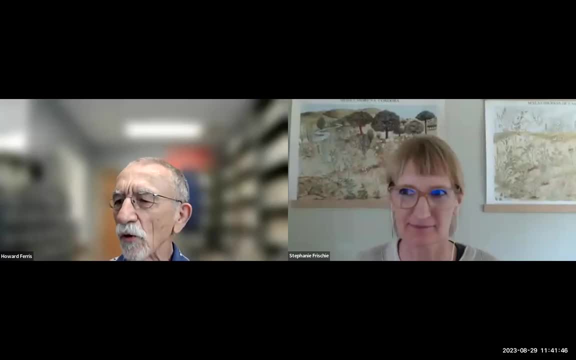 and we're looking forward to hearing about roles of nematodes in soil ecology and soil health. Thank you for joining us. Okay, so are you seeing my correct screen here? Why don't you go ahead? I had to stop my share And now, if you can, go back to Zoom. 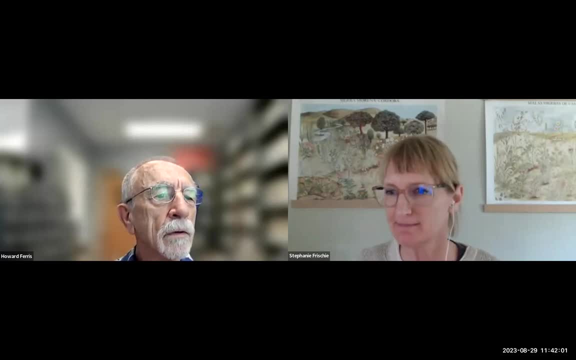 and find the green share screen button. Okay, so Sorry about this. I know you had me practice this, It's all right. All right, There's lots of little things on my screen: Go taskbar. Okay, Maybe that's it Okay. 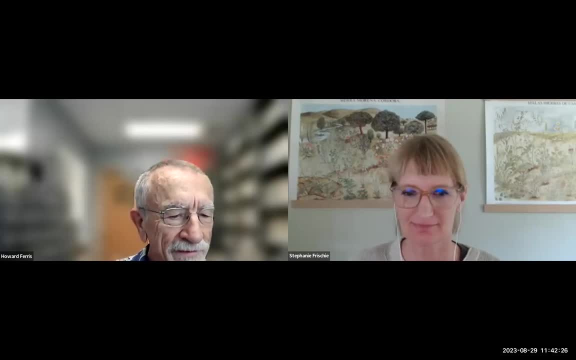 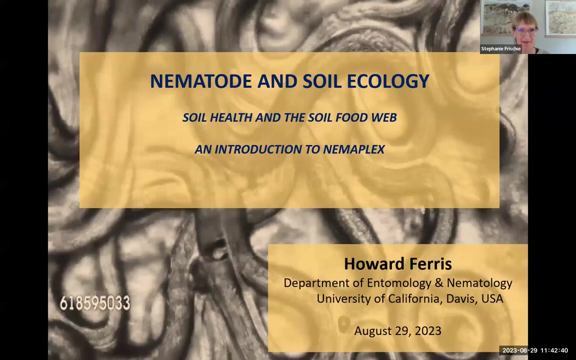 Let's go to Zoom And I see you. Okay, so now I'm going to share screen And then you'll get a choice of what you share, and your PowerPoint presentation should be among those choices. That's it. It's coming up. Yep, There, You got it. 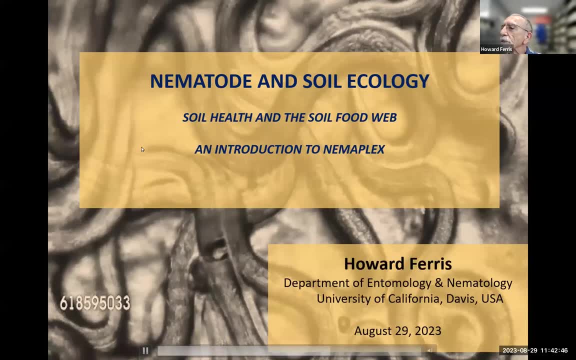 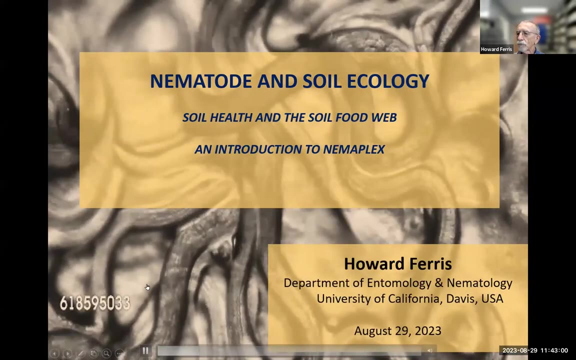 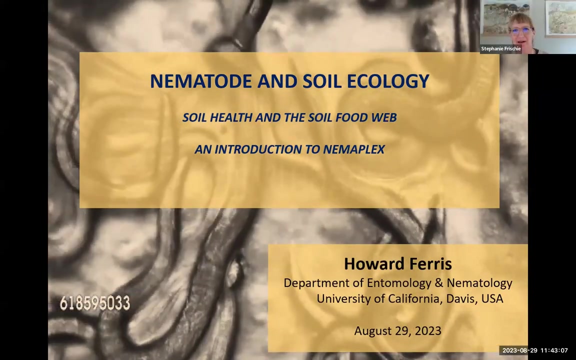 Okay, Are we on the? and we're on the right page here. huh, We're on the front page, Mm-hmm. Okay, So I need to start with the delay. Yep, The video's moving now. Okay, There we go. 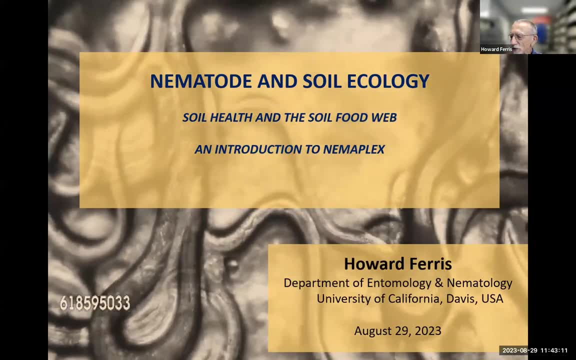 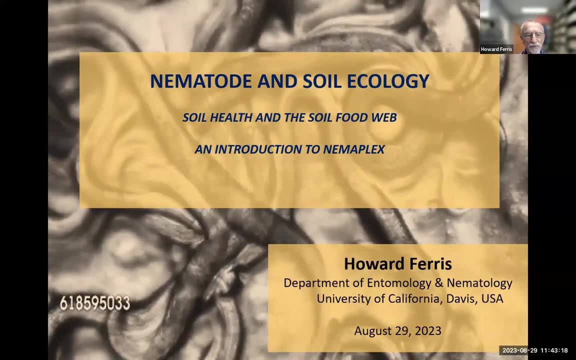 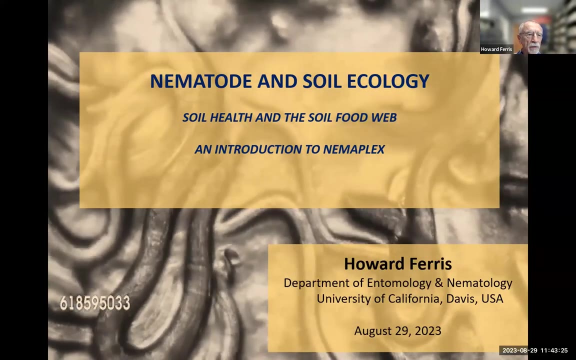 Yep, Got it Okay. Well, thank you very much. It's been very interesting this morning Listening to all these presentations and the kind of overlap of principles and philosophies that that's read all the way through them. So I'm going to talk a little about the role. 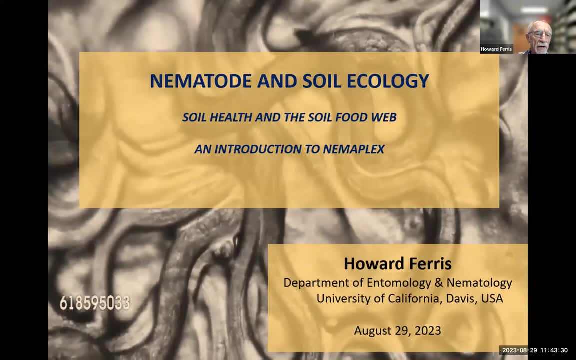 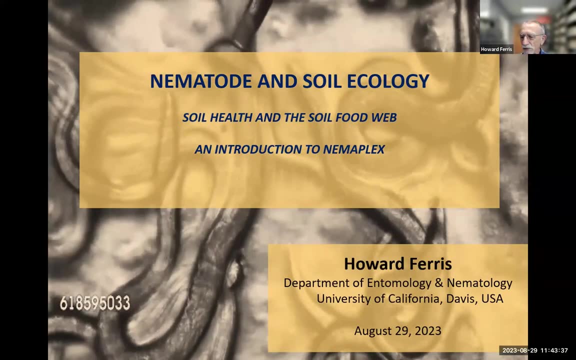 of nematodes in soil ecology and their impact on soil health and the soil food web, And if we have time I'll introduce you to the NemaPlex website. So first of all, just a little about wait a minute stop. 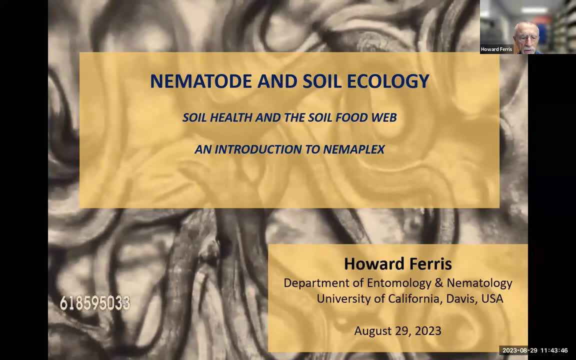 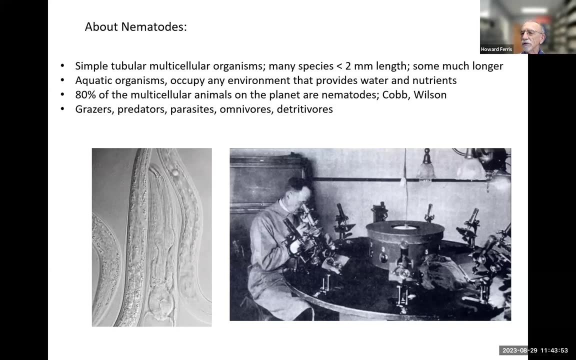 NemaPlex. Okay, So first of all a little about nematodes And, as you heard in the earlier presentations, nematodes are simple multicellular organisms. Most of the species that are in soil are probably less than two millimeters in length and a lot of them less than one millimeter in. 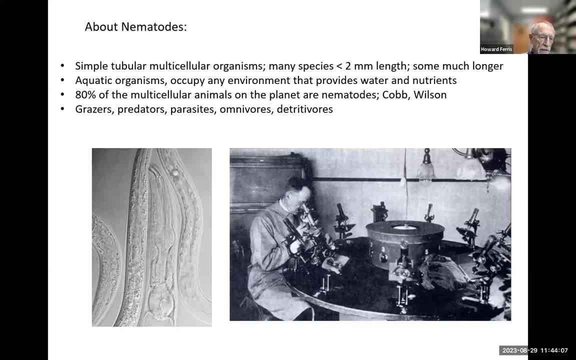 length. They're aquatic organisms. They live in the water films around soil particles, And so for activity, they live in the water films around soil particles, And so for activity the soil must be moist, but they can certainly tolerate dry soil and go into an anhydrobionic. 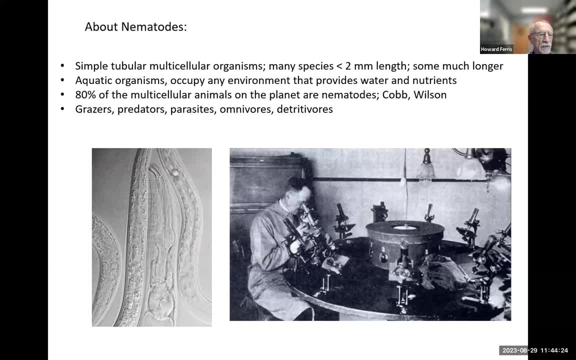 state from which they recover when the soil becomes moist again. They occupy any environment that provides nutrients and water, And we've talked a lot about, or heard a lot about, the abundance of soil organisms and organisms generally this morning, But it's estimated that 80% of the multicellular animals on the planet are nematodes. That's not 80% of the species. 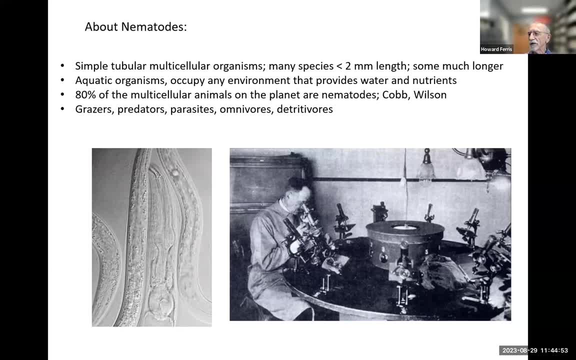 of course, but of the individual multicellular animals are nematodes. Now it's pretty hard to prove that, but it's left based on observations of abundance of nematodes by people like, for example, Cobb here- And Cobb was a fellow 130 years ago, sometimes called the father of. 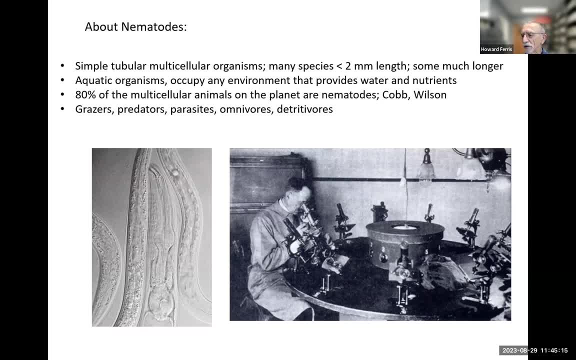 nematology In the United States. among other things he described in one paper described 100 species of nematodes And by doing that he had technical helpers working at these various microscopes setting up slides with the nematodes he was interested in identifying And then they could. 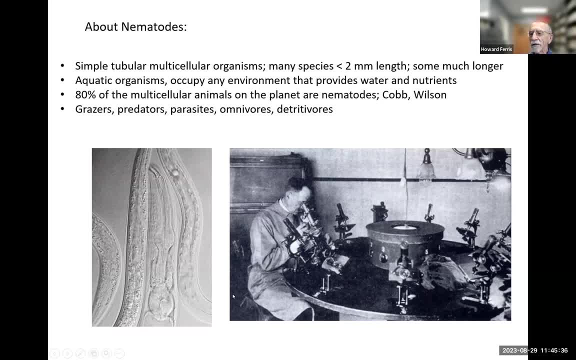 rotate the table around so that he could get on with the job of doing the identification. And I'll talk a little about Wilson later. Dr William Shepard, Nematodes generally fit all kinds of feeding habits: grazers, predators, parasites, omnivores. 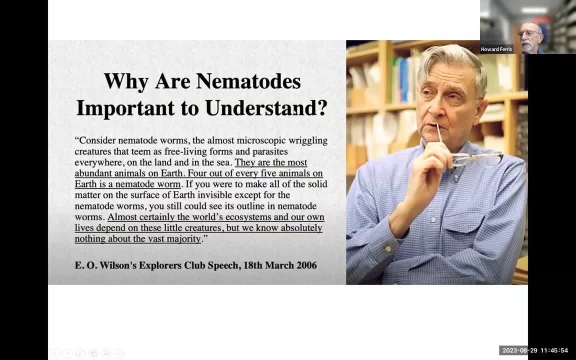 tritophores and so on. And so back to EO Wilson. EO Wilson recently died, a couple of years ago, but he was a professor and entomologist at Harvard University and worked a lot or thought a lot about biodiversity generally And so, but in the in later years he became 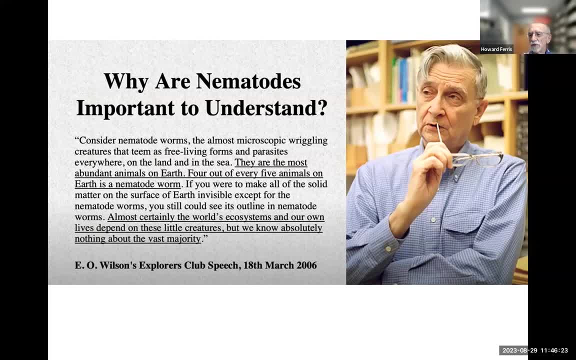 intrigued with nematodes. And so why are nematodes important to understand, He said. they're almost microscopic wriggling creatures that teem as free living forms and parasites everywhere on the land. They're the most abundant animals on Earth. Four out. 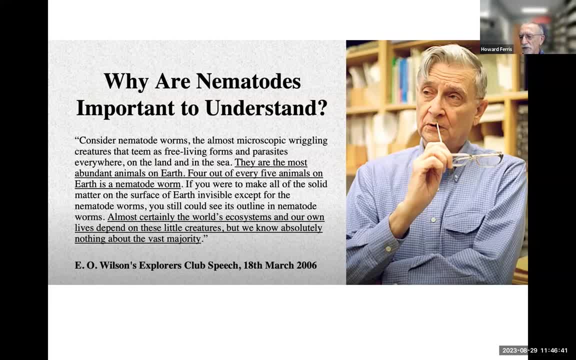 of every five animals are nematode And it went into study And then the study came out. it's a really good study. And then there were many great discoveries And we were told, say that if you remove all the solid matter on the earth, you'd be able to see the- uh, the outline of 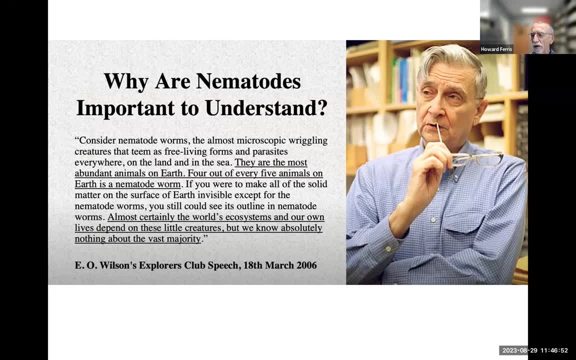 the plants and animals that have been there, and perhaps some of that, how the land had been managed by the, the uh, the types of nematodes that were there. and so he indicates that almost certainly the world's ecosystems and our own lives depend on these little creatures, but of course on many other. 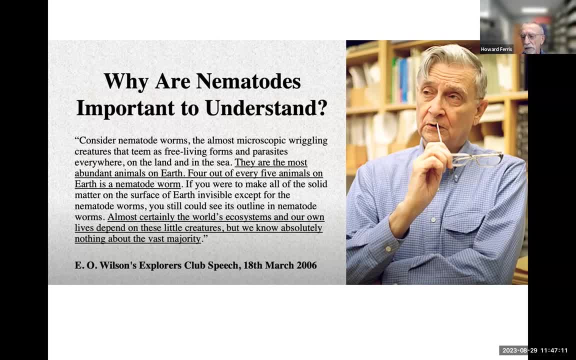 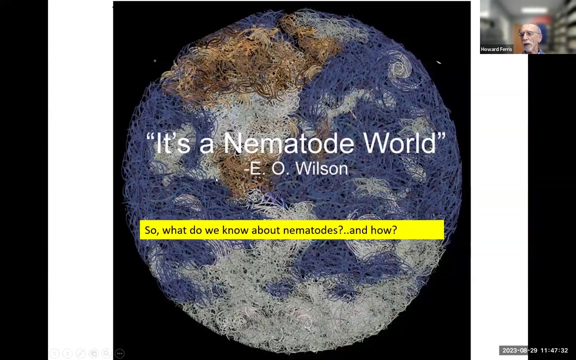 creatures that are interacting, uh, with them. uh, actually, some of that language that, uh, that wilson used was, uh, originated with the top 130 years ago, uh, who was sort of quite eloquent in his detail of the abundance, importance and diversity of nematodes. so, but following on with wilson, here, uh, we say it's a nematode world. so here's the planet. 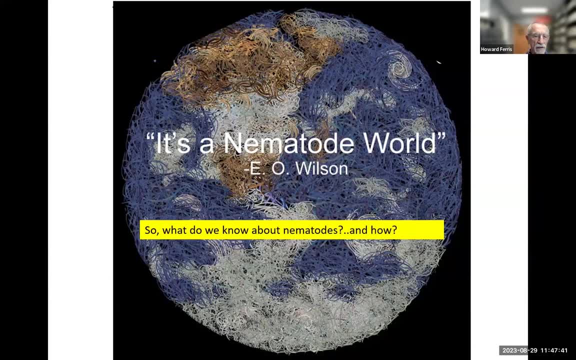 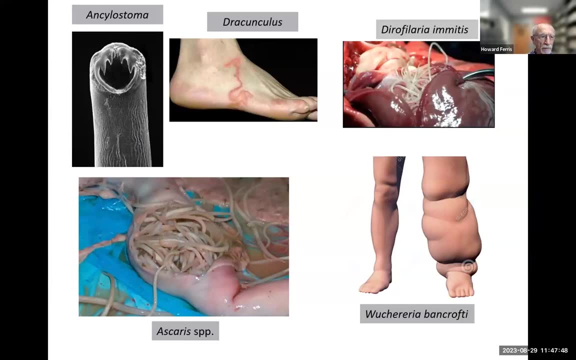 mniej mean with nematodes. but what do we really know about nematodes and and uh, how do we know it? well, we know a lot about nematodes that are that affect us directly, right, parasites of humans and domestic animals. so, for example, hookworms that might be carrying into the surface mucosa of the 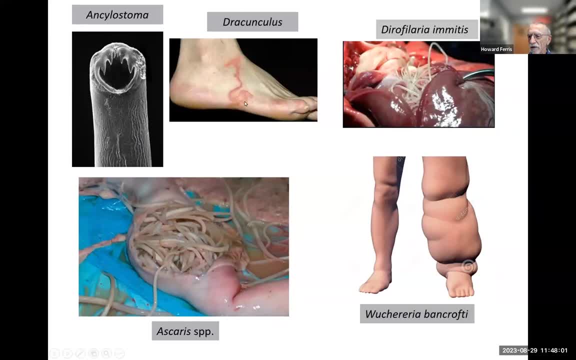 intestine or guinea worms here under the under the skin. uh, we know, for example, uh dog hard work And most dogs receive some kind of treatment or anti-helminthic treatment to control dog heartworm. We know a lot about nematodes like Ascaris that are intestinal parasites. 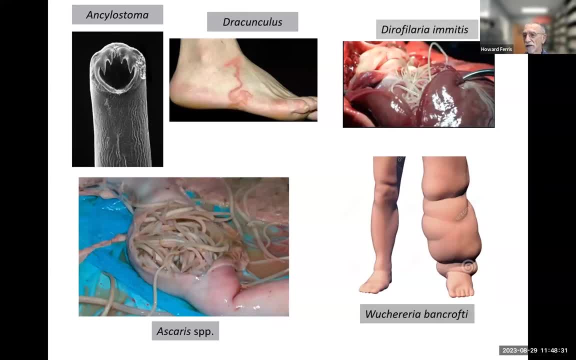 And I talked about nematodes in soil being less than two millimeters in length. Some of these nematodes are 30 centimeters in length And, of course, here's elephantiasis attributed to wujiraria, which is affecting the lymphatic system of the human. 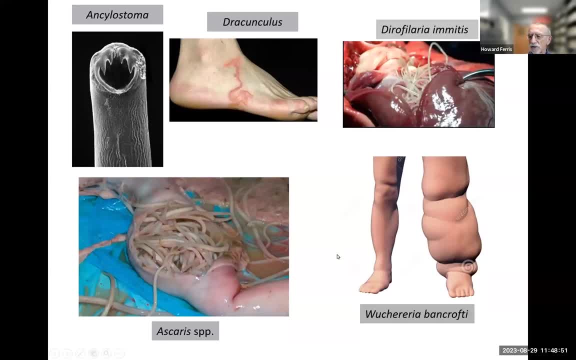 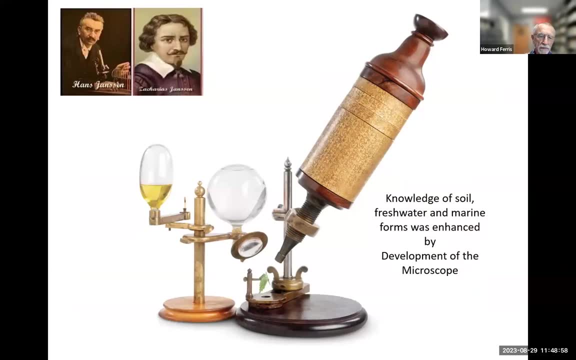 So these are diseases that have been known for a long time and studied for a long time, But really it took them through the development of the microscope for us to increase our knowledge of soil and freshwater and marine forms. So this is three or four hundred years ago. 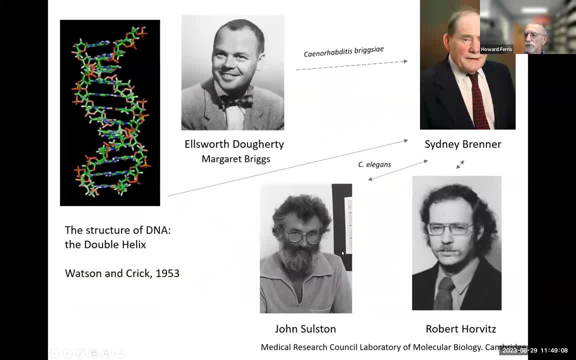 Both of the Janssens were developing primitive microscopes, And so that gave us the ability to look at these nematodes. The next thing I think that was important in terms of small soil nematodes goes back to Watson and Crick and the structure of DNA. 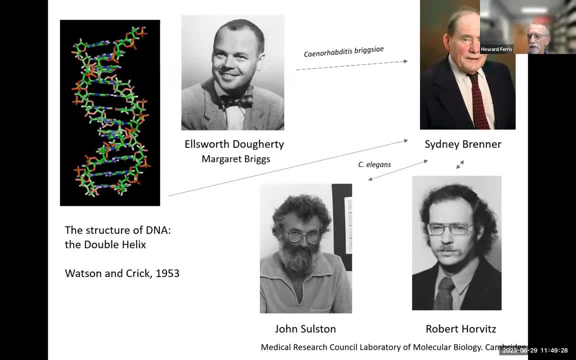 So Watson and Crick and of course Rochelle and Franklin, developed the structure of DNA And shortly after that, perhaps in the 90s, we had the first nematodes, And we had the first nematodes, And we had the first nematodes. 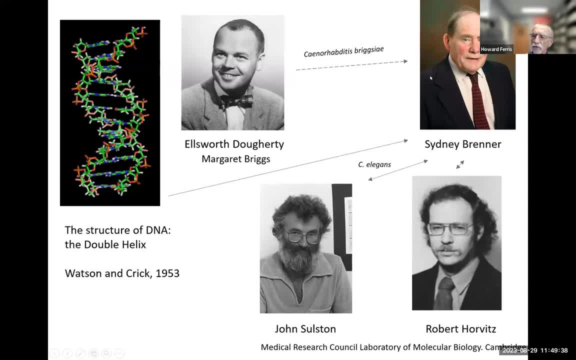 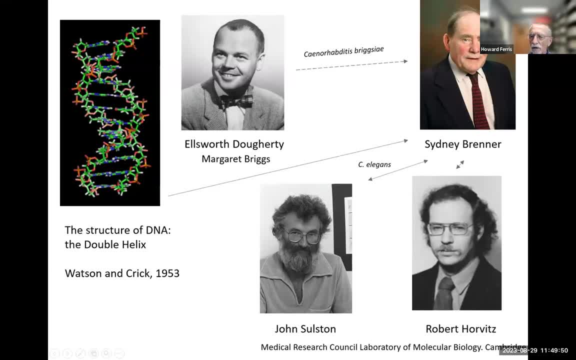 How does a double helix translate into an organism? What is it that – what's the transfer And how does that happen? And he happened to be visiting California and he ran into Ellsworth Doherty. Ellsworth Doherty worked at the Kaiser. 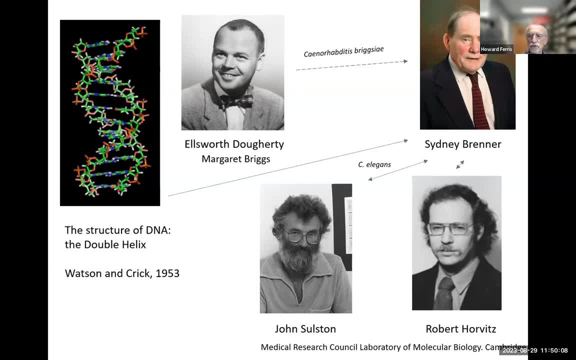 He worked at the Kaiser Research Center in Oakland, but he also was an associate – had an associate professor position at the University of California, Berkeley. Well, Doherty was an expert on red-digit nematodes, the red-digit nematodes of bacterial feeders, and he had worked extensively with them. 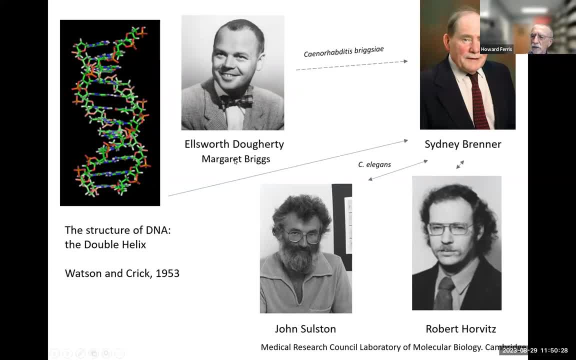 He had a graduate student, Margaret Briggs, and Margaret Briggs took soil samples in the Stanford Forest, So the forest at Stanford Stanford University in Palo Alto, And there Briggs and Doherty described senoreptitis briggsii And briggsii – senoreptitis briggsii is an important nematode because it's hermaphrodite, but under certain conditions of temperature it will also produce males. 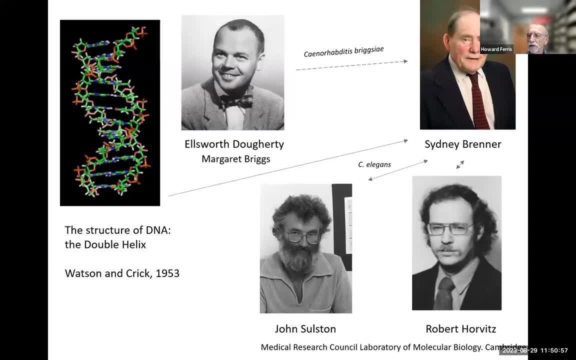 So they could do sort of mating experiments and see how the offspring and mutations and variants pass through the population. Well, so Doherty told Brenner about that and Brenner was intrigued. He went back to London and did some sampling and found a related species, senoreptitis elegans, which became the biological model for developmental biology. 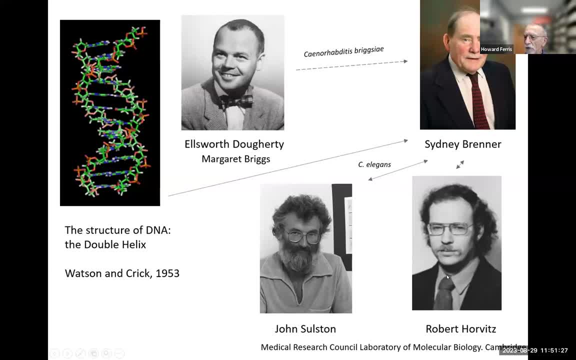 Working with Brenner, with John Solston and Robert Horvitz. all these guys got the Nobel Prize for the work that they were doing here. Solston was a particularly interesting guy. He was a very interesting guy. He was a very interesting guy. 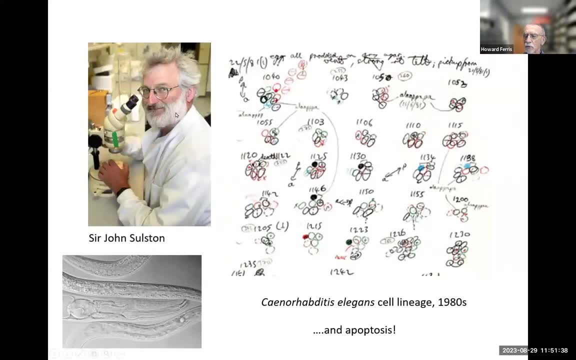 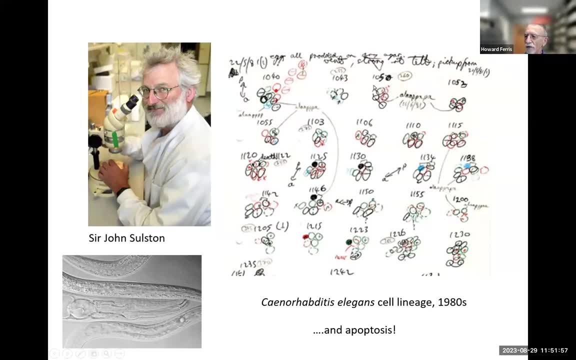 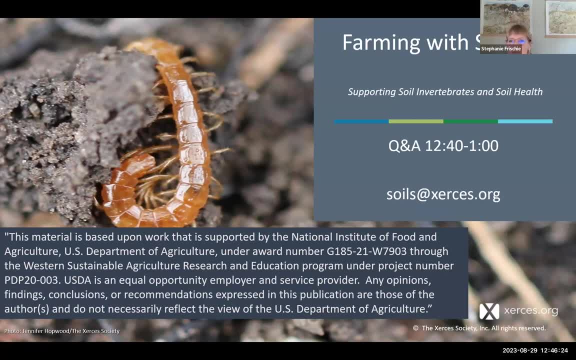 So, and of course I can't identify what he was doing here with these sketches, but he was able to trace the cell lineage of every cell. Howard, do you have anything else to add? Well, just in terms of was working on the защищance language. 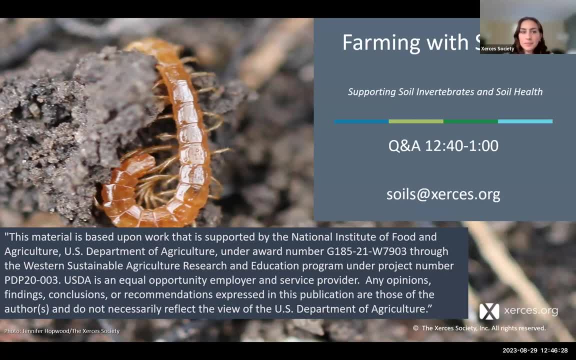 itahh well, just in terms of was working on the защищance language. itahh well, just in terms of was working on the защищance language, especially with pneumatites, Especially with pneumatites. 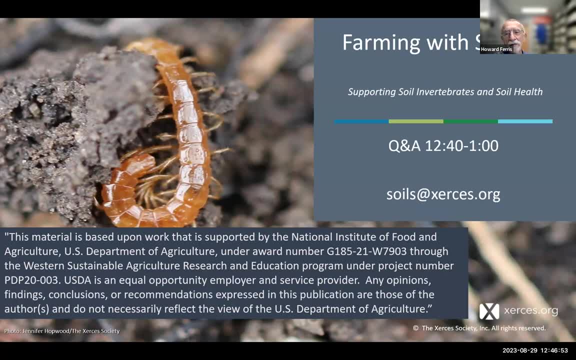 In other words, you can apply repeatedly, For example in orchards, without causing damage to the trees, but to reduce the nematode. you realize they're not having an impact on the nematode community anymore, So the evolution of resistance does occur. 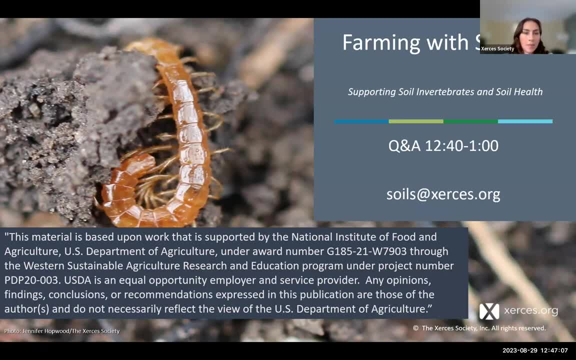 Great. Another question for you, Dr Farris: Are there nematodes that eat wireworms? Probably not eating them directly, but there are nematodes that we call entomopathogenic nematodes that have inside their body a capsule of toxic bacteria. 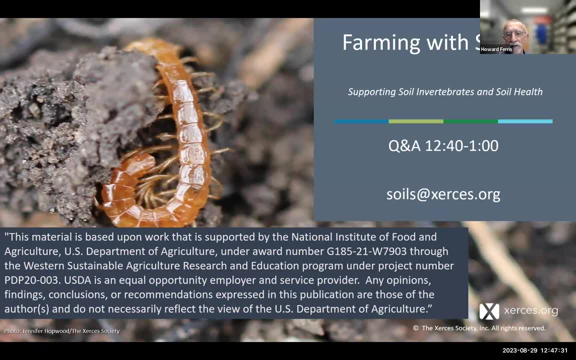 And so, when they attack an insect, for example, they release the toxic bacteria. The toxic bacteria kill the insect, grow on the dead body and the nematode feeds on the bacteria and the dead body feeds on the nematode. 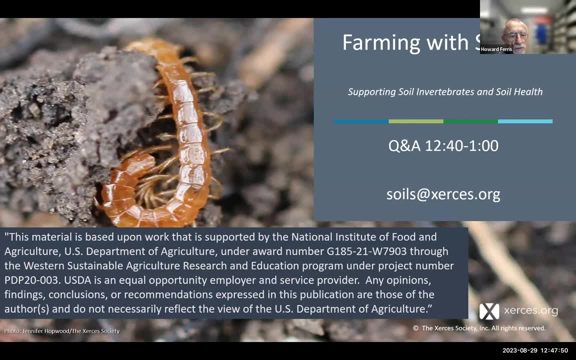 So I imagine that would happen with wireworms as well, but I don't know of any examples. Thank you. Next question, another general one. I've heard people say that alley cropping, et cetera, compete with the cash crop for available water. 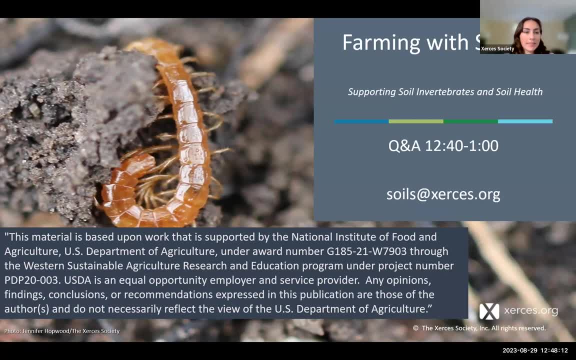 How significant is this competition? Does it balance out with the benefits to soil, health cover, OM, et cetera? I can take that one very seriously Very quickly. that's a good question and it's certainly a valid concern. 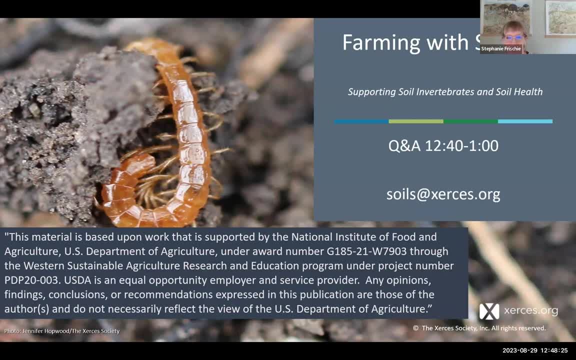 But I think, as far as being able to say how significant the competition is really, there's no one answer for that. It varies a lot on the climate of the area, the soil type, the crop type, the particular weather of that year. 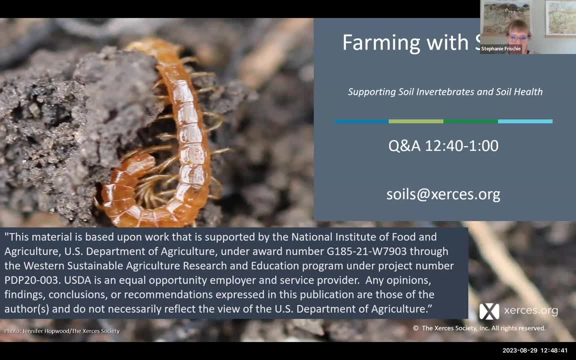 I'm familiar with some examples from Mediterranean climates, with olives in particular as the crop And then using the winter annuals as the alley crop or cover crop. So those are the nests that are not really competing for water during the summer, when water deficit would be at its peak concern. 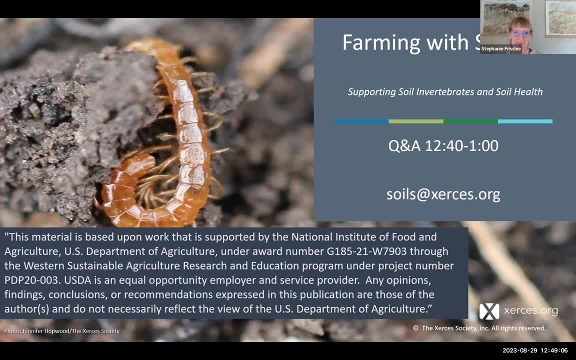 So, yeah, good question, but I think it really varies case by case. Got it? Another question: More farmers are using brassica cover crops to control nematode populations. can you speak to the benefit of this biofumigation functions? 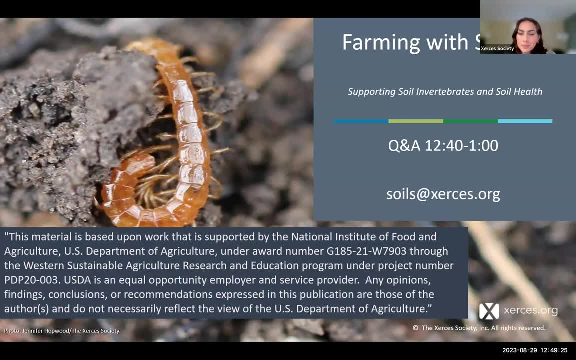 and the possible impacts on beneficial nematode species. Yeah, it's a good point. Yeah, so biofumigation is an important and emerging strategy. Often it's more effective if there is some kind of a tarping system, for example in greenhouses and so on. 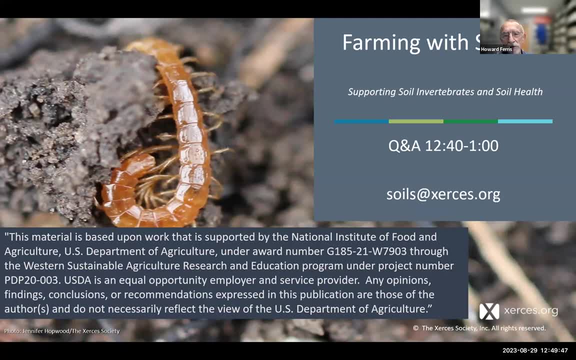 But definitely. we've seen, you know, effects in the plant parasitic nematodes related to brassica cover crops. Now what impact does it have on non-parasitic nematodes? I think that the bacterial and fungal feeding nematodes are sufficiently resilient. 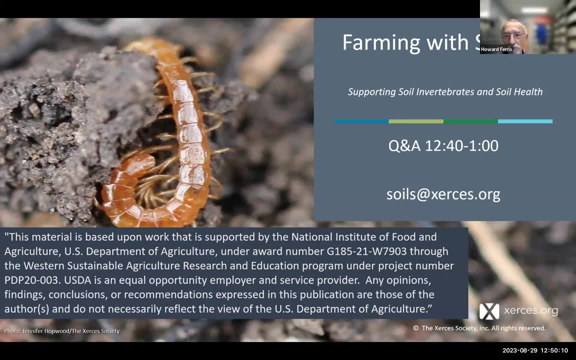 that they would recover very rapidly if they are impacted. But I sort of have a feeling that the predator, the larger predator- nematodes- would be impacted. But I don't know that and I don't know that anybody has really done that study. 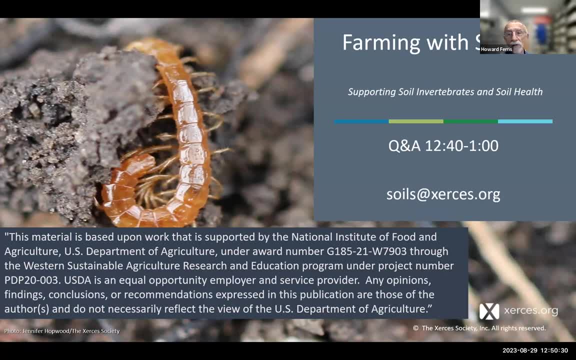 I mean, it's an important, important issue. I don't think we have looked at it thoroughly enough. Great. Next question: Any comments on biochar? Go ahead, Dr Ferris, if you have any. Yeah, thanks. 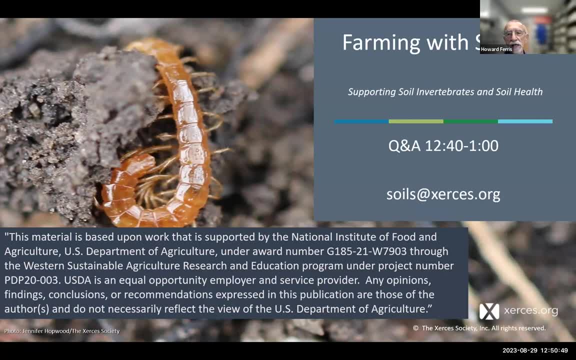 You know we've thought about it a lot. I don't see any evidence of benefit in terms of nematode management. I mean, there's been a lot of thinking about it, but in terms of experimentally related to nematodes. 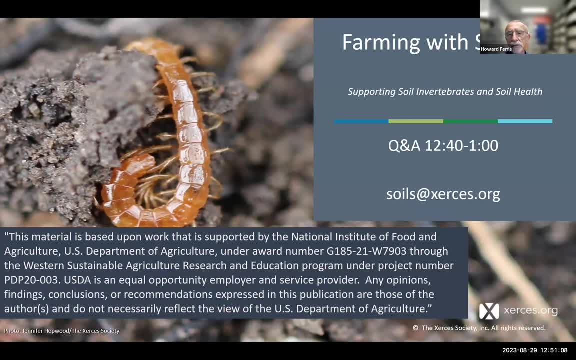 not really much has been done, So, on the other hand, I think that any way of incorporating carbon into soil is a good thing. So how do you put it in? You put it in if it's in biochar form, or you put it in pre-biochar. 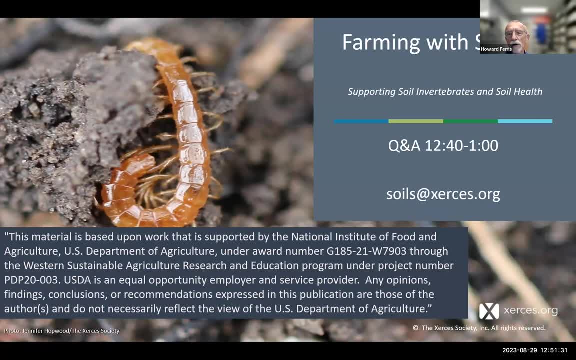 but I think always it's a good thing to get more carbon into the soil. We have depleted carbon in the soil in agricultural systems. Here in California we're looking at 1% organic matter and we look at the, the surrounding areas of those fields and it's 2% or 3% organic matter. 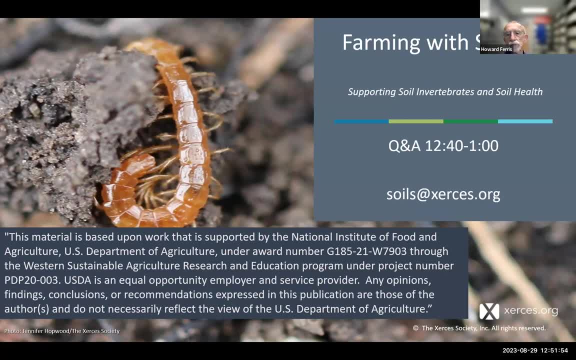 And it's difficult to get that percentage up. Good, Okay, We got through all the questions. Thank you, Raven. Thank you everyone for posting those. I think we've got eight or so minutes left and it would be great to have you demonstrate the website, Howard. 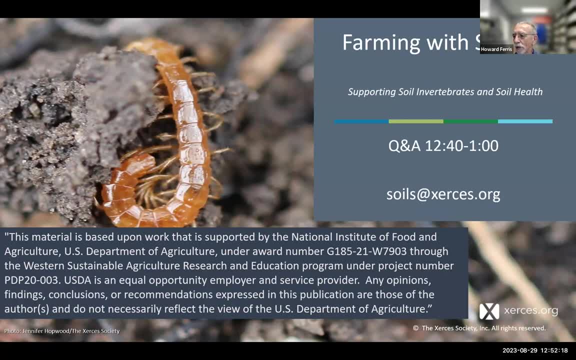 Well, I just I'll just show you a little. now I'm going to make sure We'll have to have you go back and do that screen sharing. Okay, Hang on, let me do this screen sharing, So that's. 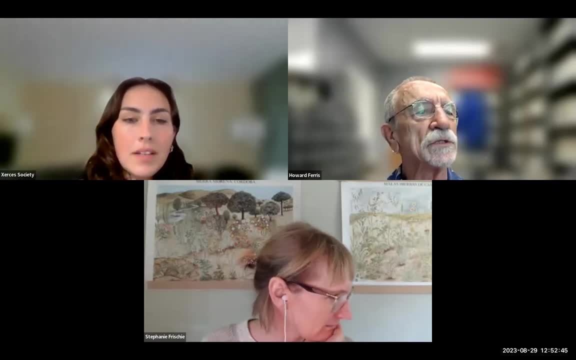 So you're going to tell me how to do that again, because I don't see anything that says screen sharing. I know you've told me a hundred times: don't pass the bar. There we go. Good, You can see our faces. 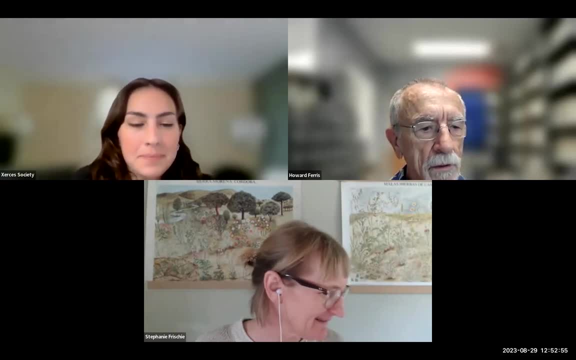 We go to here, And now we go to share screen, Yep, And now we go to. Which one am I looking at? I'm looking at this one here. I think There, it is Okay. And so here's where I was and here's where I was. 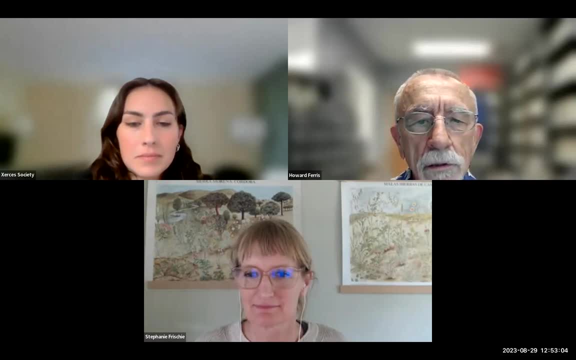 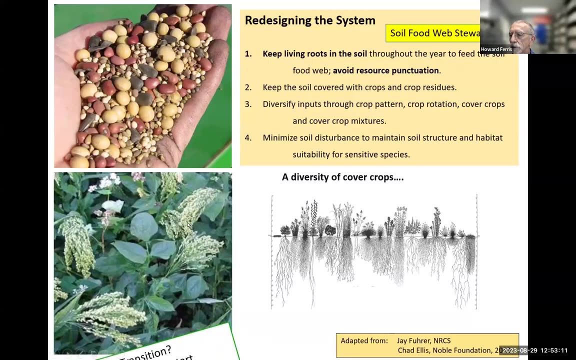 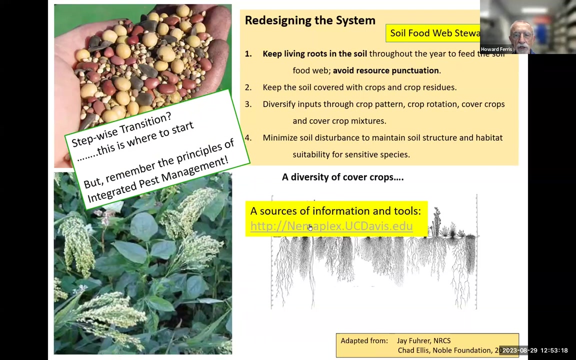 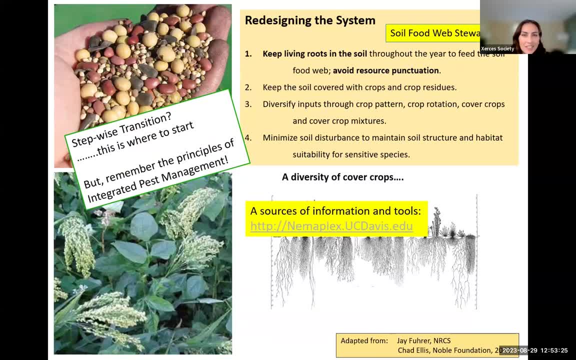 Now I'm sharing. Yeah, you'll have to reshare it, So go out of sharing. Okay, Thanks a lot, So stop sharing the screen. New share, Yeah, new share. Okay. Now, this time, choose the website as what you share instead of the PowerPoint. 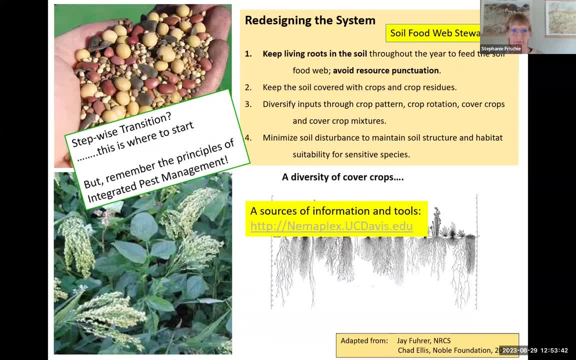 That's where we lose you. It doesn't make the jump. There it is Again. I show you're not seeing my website, right? You'll have to stop share because we're seeing the PowerPoint, So stop sharing that, Sorry so. 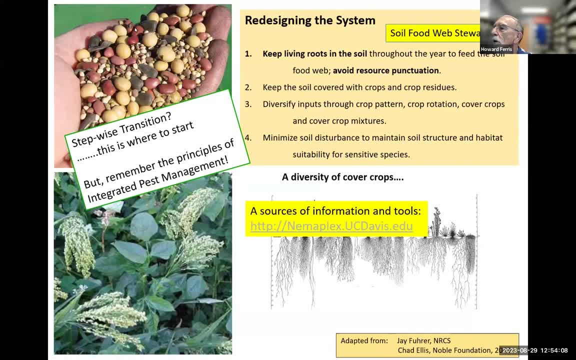 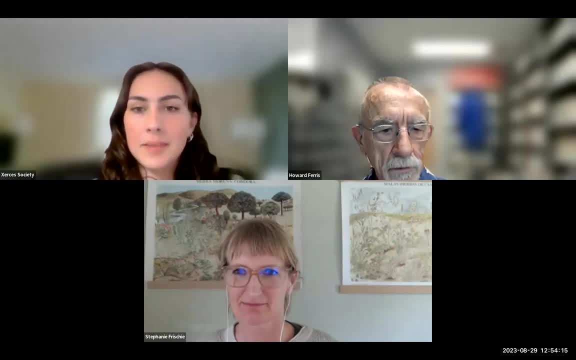 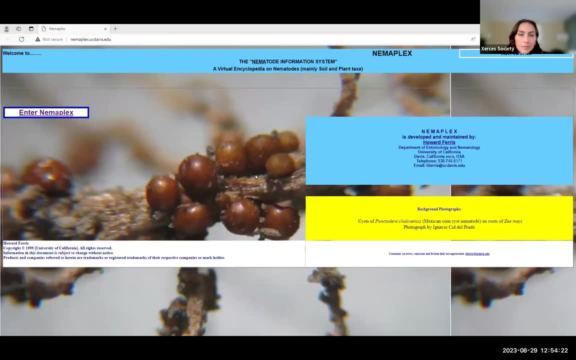 The video up here. Oh, up here. I see Right, and then reshare, but choose the window with your website on it. Yeah, you can see it. Okay. So what I want to do is Nemo Plex is a website that essentially it's like my. 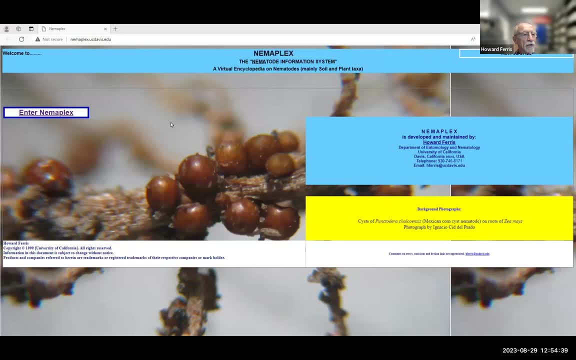 stamp collection. you know, I said when I get older I'll have a stamp collection. well, actually I started this when I was younger, But the idea is that everything I ever wanted to know or ever knew about nematodes- 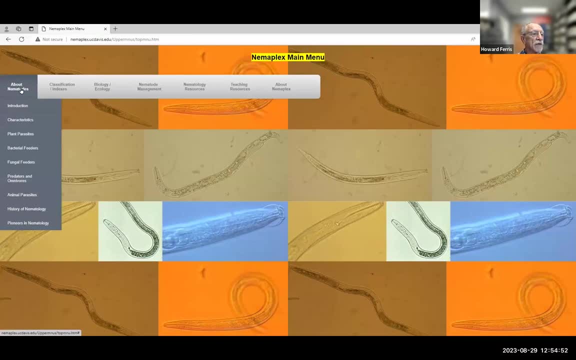 So I enter Nemo Plex and there's all kinds of things about, you know, types of nematodes and their biology and behavior, and history of nematology or classification and biology- But what I really wanted to show you today- and there are some teaching resources- but what I really wanted to show you today- 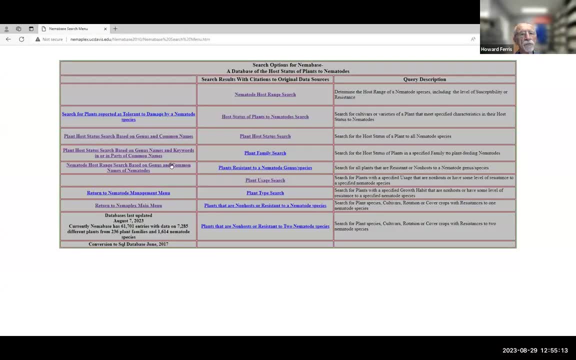 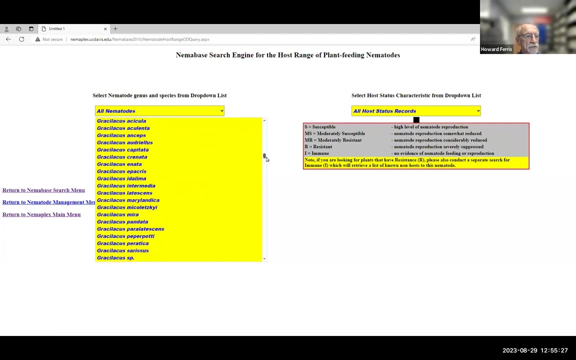 was Nemo base, and Nemo base is a database of the host status of plants to nematodes And I have it set up to where you could select a nematode. For example, you could have all nematodes or you could say I want to take one. 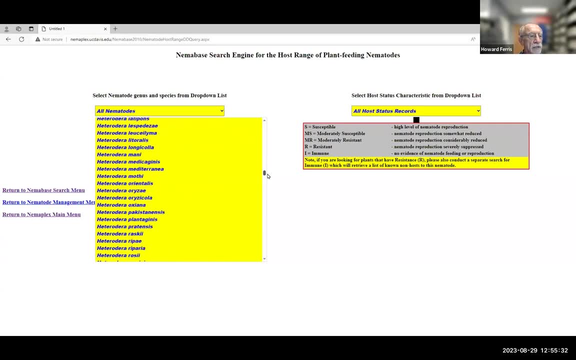 like say haplolimus, so I can get there. So we'll take haplolimus columnus. So haplolimus columnus. This is what's called a stunt nematode. The plant parasite impacts cotton and soybeans. 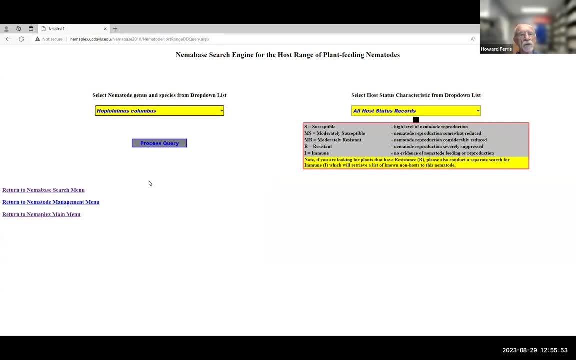 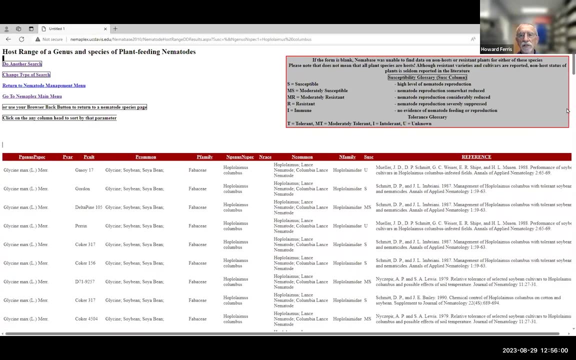 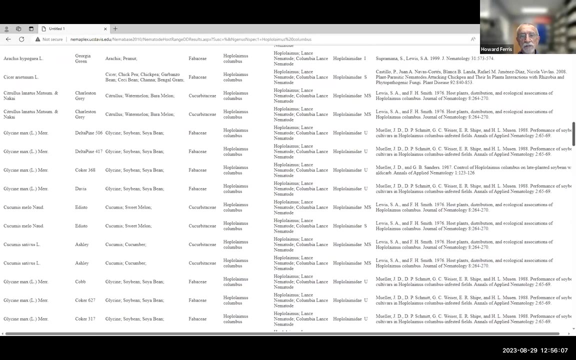 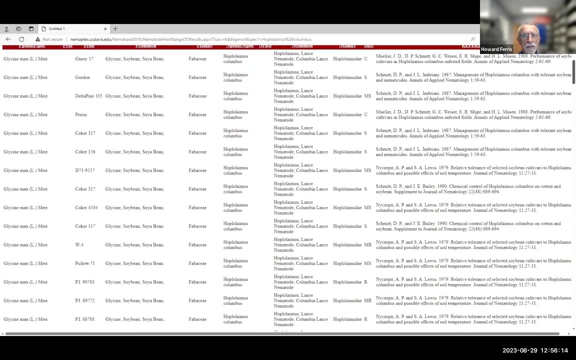 Important in the Southeast United States And we'll say all host records. So I want to find out what species. So now, what's telling me all of these, all the known literature on plants that are resistant or susceptible or have been studied in any way to haplolimus columnus? 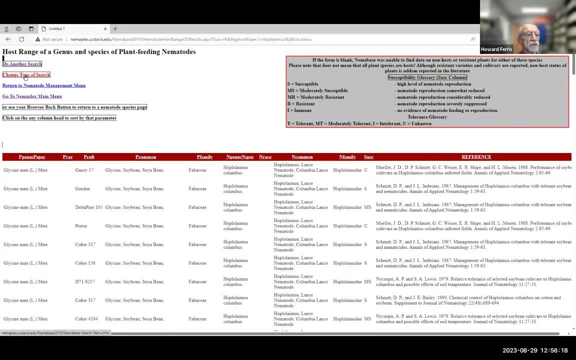 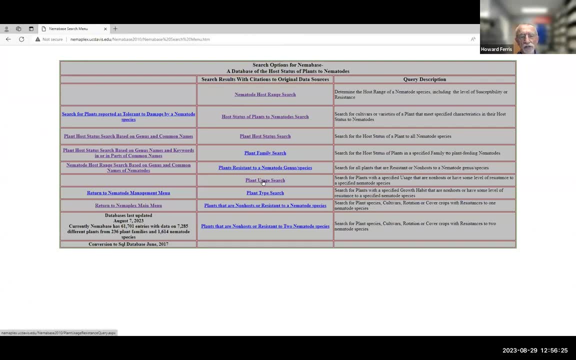 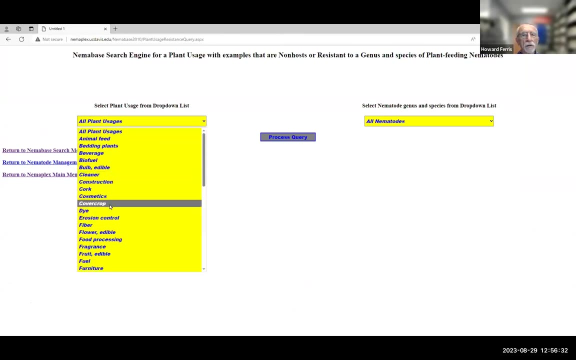 So a lot of them. Now, perhaps what I want to do is change the type of search, And maybe I'm interested in plant usage. I would like to know, for example, plants that I could use as a cover crop for haplolimus columnus. 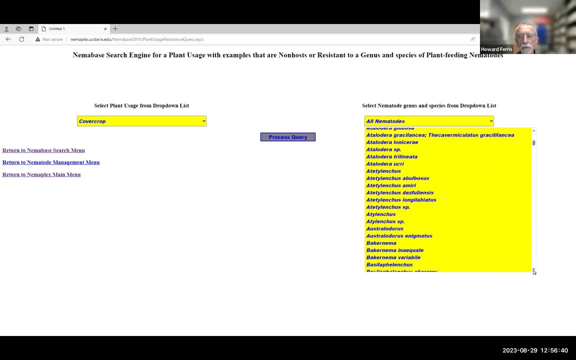 Get myself back down there. So there are lots of species of nematodes that are in here, of course. Probably wasn't all that wise of me to select the haplolimus columnus, especially not that. well, let me select another one. 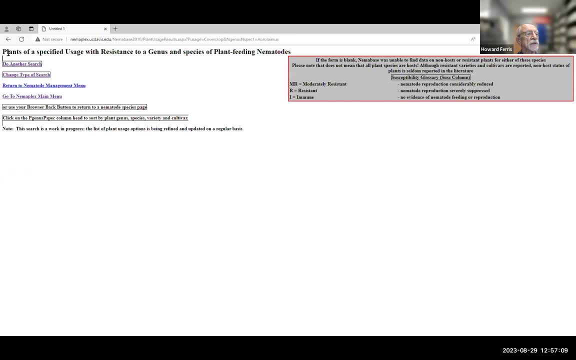 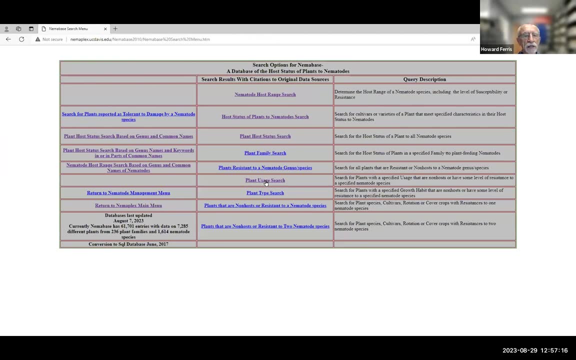 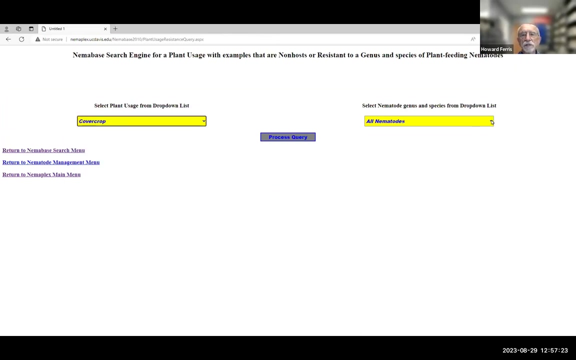 So I'll select this one. Of course I selected one. I'm going to change the type of search, And so I was interested in selecting a cover crop with resistance to. part of the problem is that you guys have got your faces right in the middle of my. 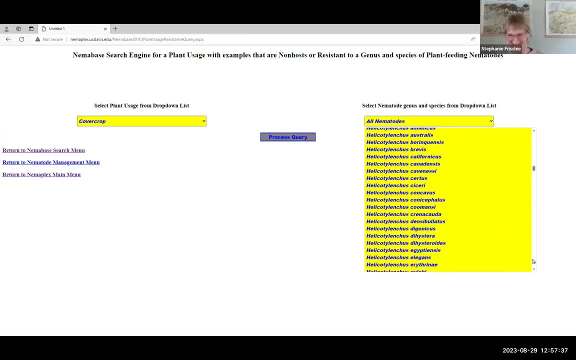 Sorry about that. No, they're very attractive faces, but it's just a. it's just the way the slide bar is coming back. Yeah, OK, so haplolimus columnus is somewhere around here. So now I'm saying I want to grow a cover crop. 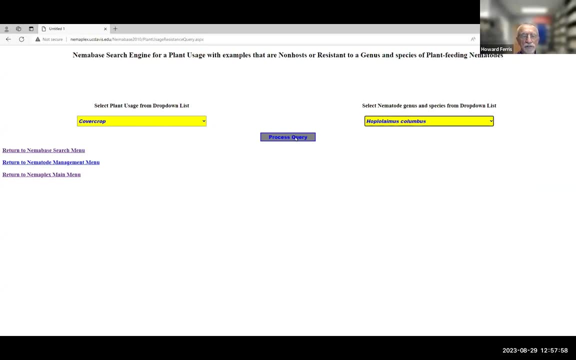 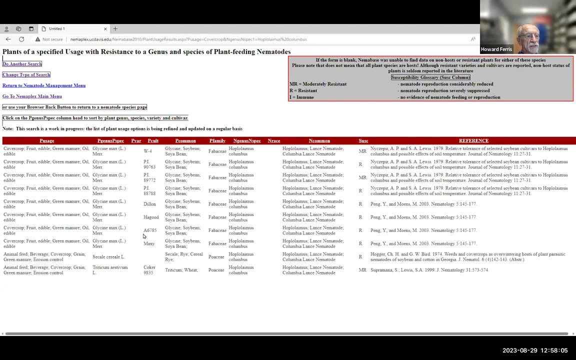 I want to know what cover crops might be available. That means they have got resistance to haplolimus columnus And so there's very few of them. And there's some varieties of soybeans they suggest might work as a cover crop: Evergreen manure. 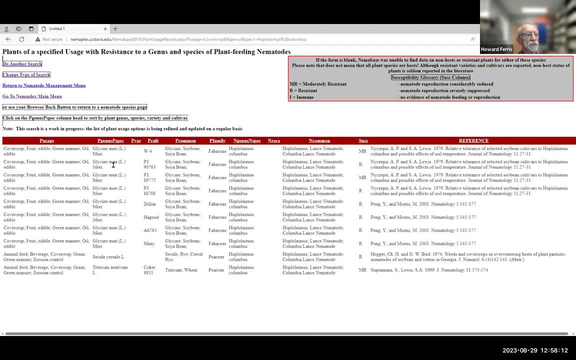 And so various species of crops that might be available. And here's if we wanted more information. notice that they're all resistant or moderately resistant to the nematode. But then let's say that we wanted to. I'm not going to take too long of this. 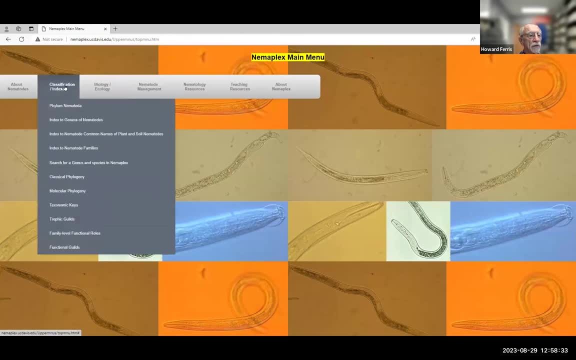 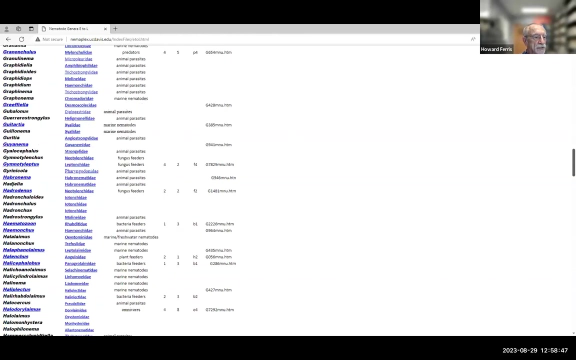 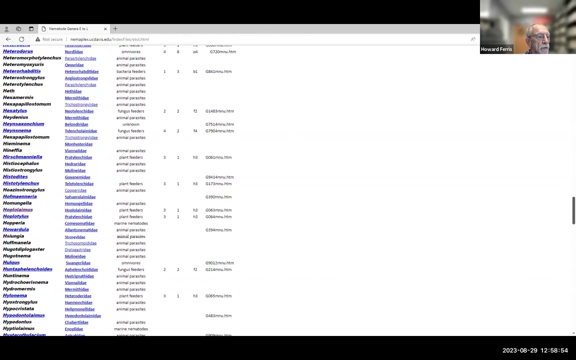 Let's say we didn't know much about haplolimus columnus. We could go down here to the index. you generated nematodes And here are all the nematodes that I have in the database, Or the ones with the G and H thing with haplolimus here. 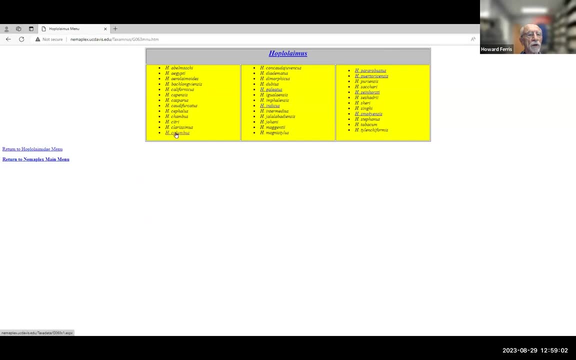 And so there are all kinds of species of haplolimus, And we were talking about haplolimus, And so the ones that are underlined or blue are ones that I have information in. So I'm just recognizing that they exist, And so we could go to the haplolimus Columbus page. 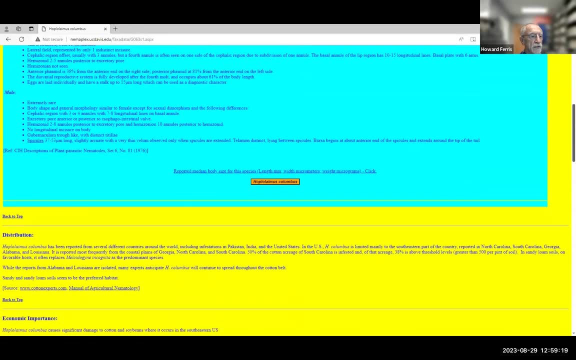 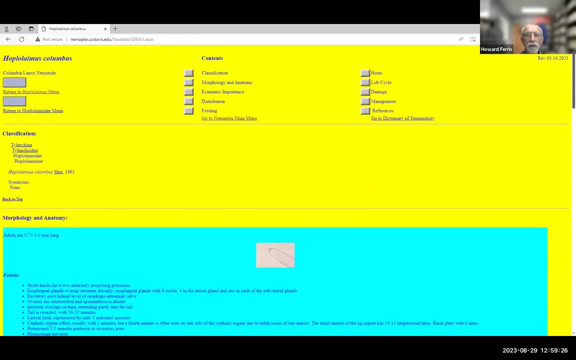 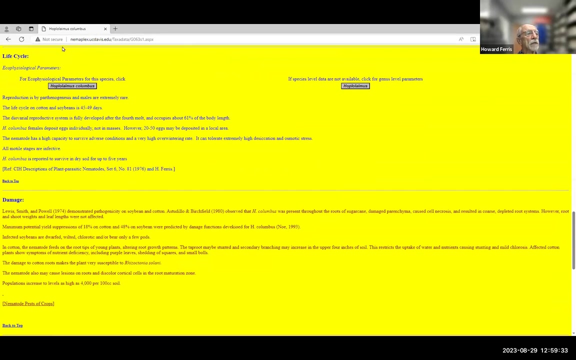 learn something about the characteristics of the nematodes, what it looks like, where it lives in the world, economic importance, its feeding habits and so on. So OK, I think that's all I need to show you about Nemaflex. 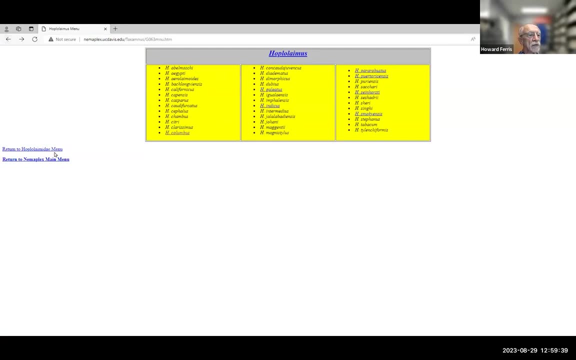 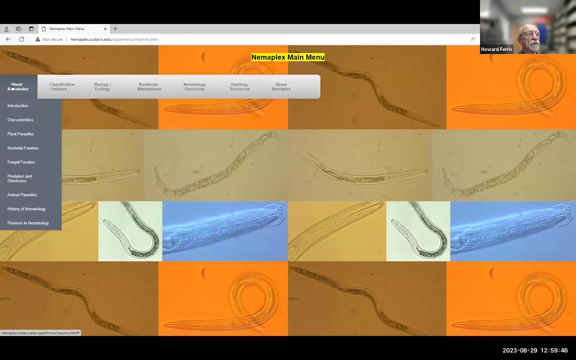 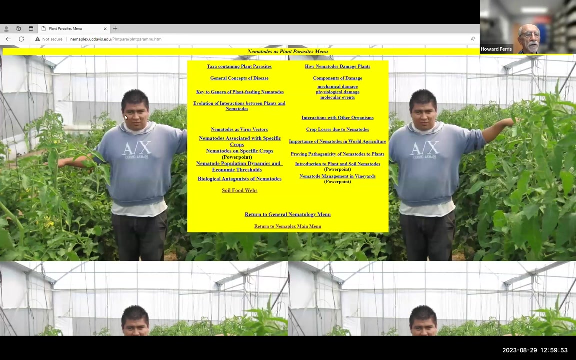 Just that it exists, and it's the kind of thing that you, if it's of any interest to you, you might want to explore yourself and all these the various attributes of it, So we could, for example, go to plant parasites here and here, my friend. 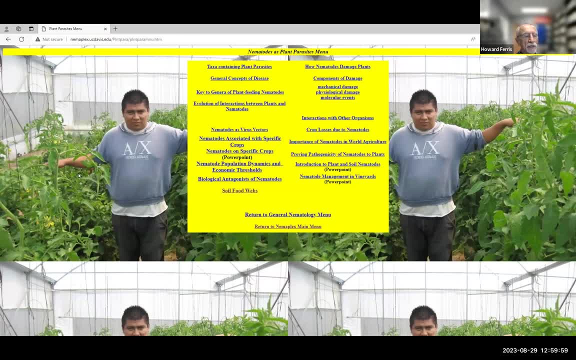 So a little sidebar here. This is a guy. I was working in Mexico with some colleagues And this guy was growing peppers And tomatoes where he was using biofumigants. So he was using actually some brassicas and other biofumigant materials. 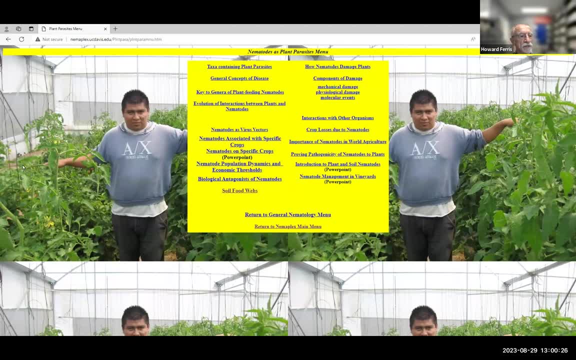 under tarp before he planted his peppers, And so he's showing you here. this hand that you can't see is showing that the peppers are two or three times higher, or 30 or 40 centimeters higher, than they were without the, without the biofumigant. 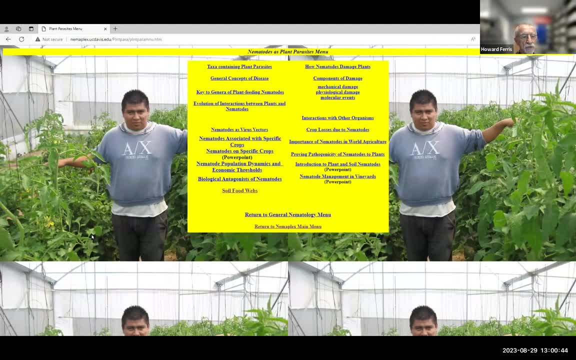 And when, when you dug into the roots, you could see very, very great differences with the populations of nematodes, the symptoms on the root. OK, enough of that. So that's, that's Nemaflex Howard. there's a new question. 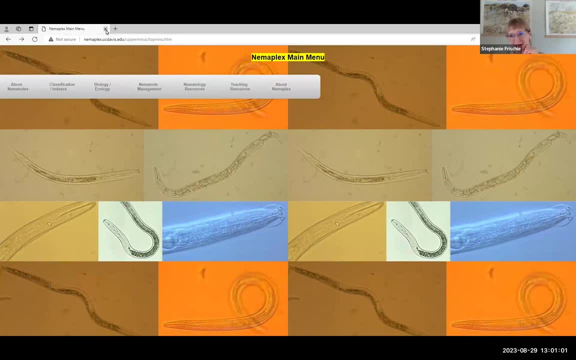 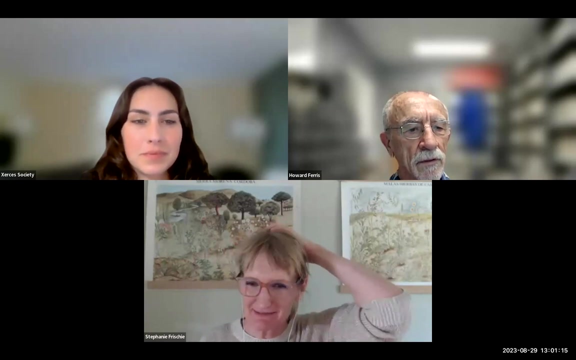 Thank you so much for walking us through some of that and for building it and making it available. It's amazing. Yeah, it's available and easily accessed, And if it's not, please call me and I'll try to make it. We got a new question for you about Nemaflex. 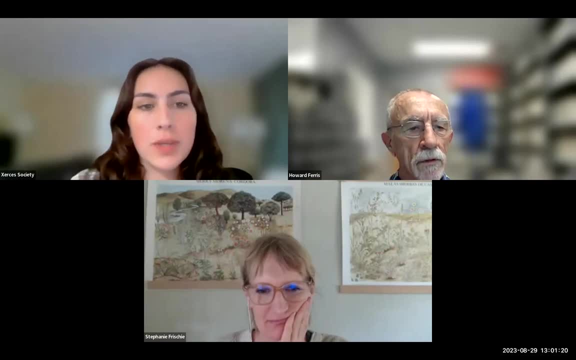 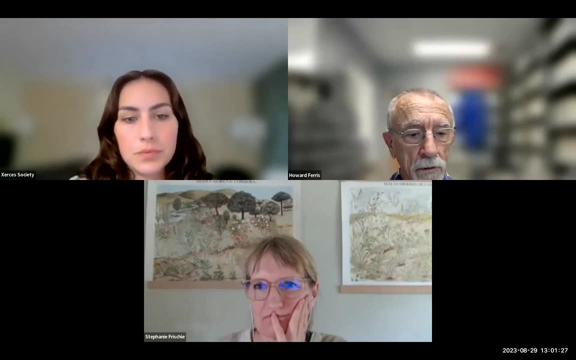 Go ahead, Raven, you would please? Yeah, of course. So which choice for plant usage would we use for perennial grasses? So which say that again, which? which? which choice for plant usage would we use to search for perennial grass? OK, so can we go back into it. 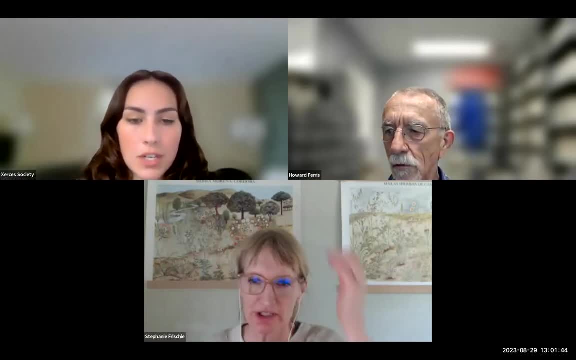 or am I out of that? So you're allowed to? Yeah, just you're out of it now. But yeah, you can go back Now. I mean no, no, You'll need to share your screen again. I wish you'd make it more proof. 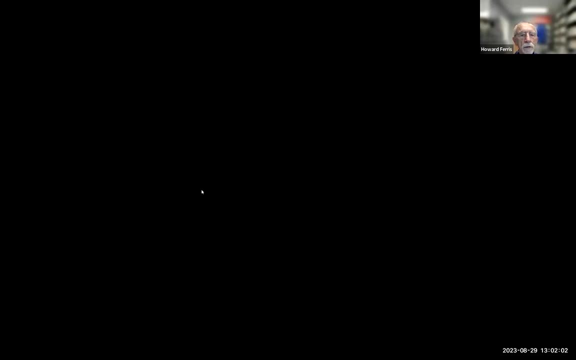 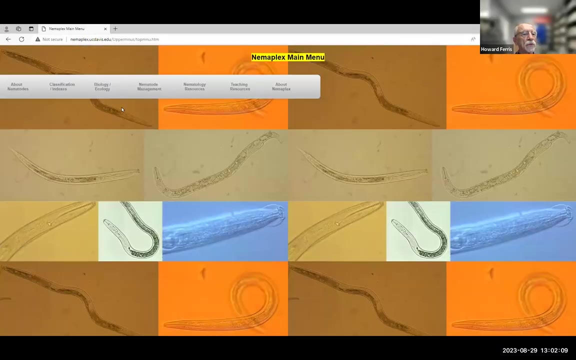 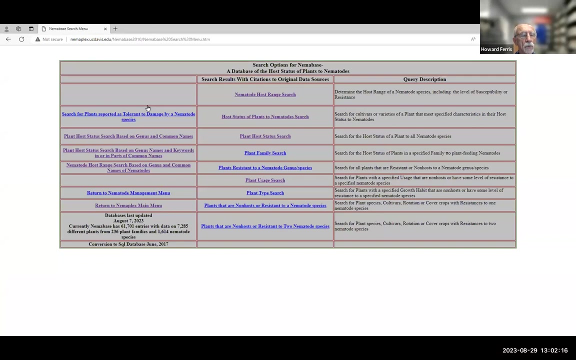 OK, Perfect, looks good at it. You got it. OK, Good, OK, so we're going to never to go to Nema base, and So we want to see what a perennial grasses that are not affected by nematodes, for example. 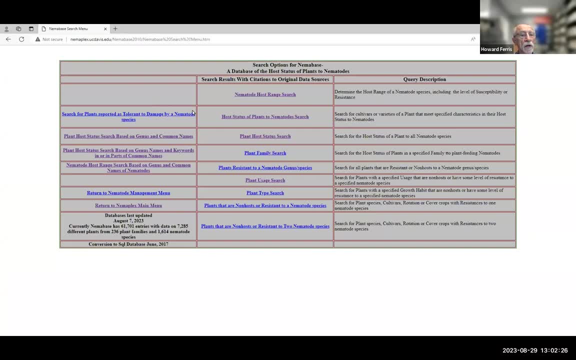 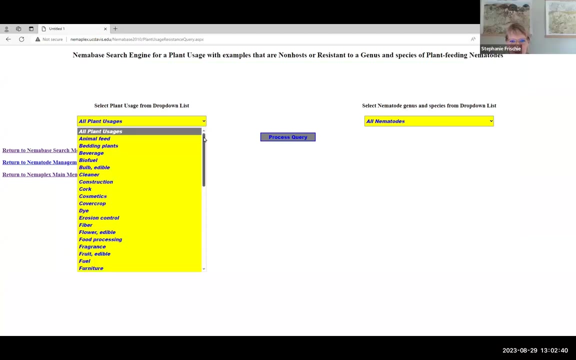 Would that be a reasonable question. Can I do that? Let's see, Because I think that I would say yeah. also, maybe the Yeah Plant usage. Is there something in the drop down menu that matches perennial grass? Yeah, so mainly they're about uses, not about plant type. 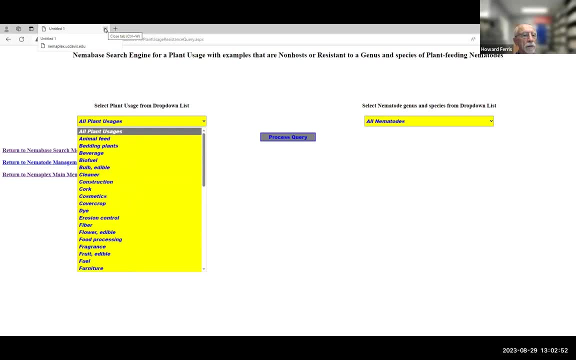 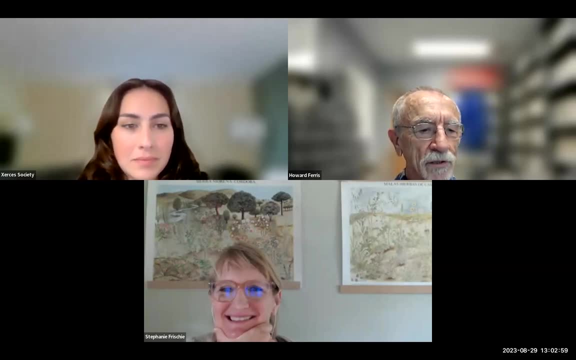 So let me go back again a little. No, I don't do that much. Your screen And I'm not back, am I Not better? We'll have to get you to reshare the screen again. How am I doing that? 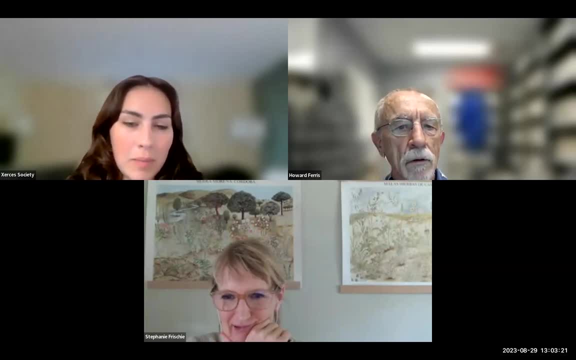 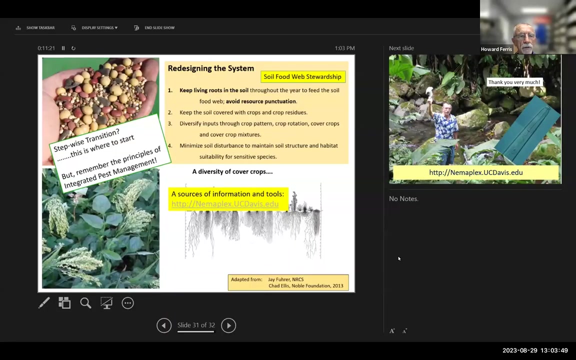 Remind me. So find Zoom and the little green button at the bottom. Oh yeah, Find Zoom. I really found the ones. Oh, show taskbar, OK, Show taskbar and Z And then share Now what? So now you're on your presentation. 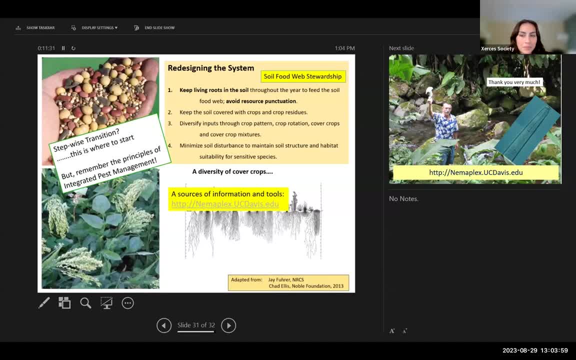 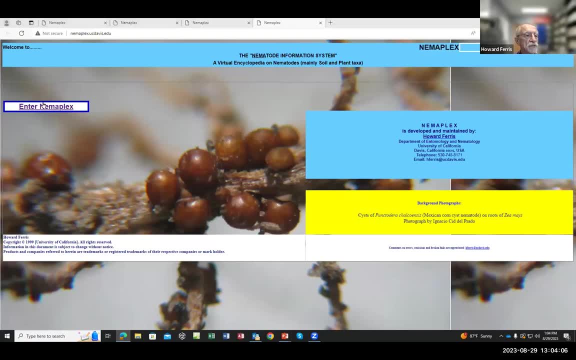 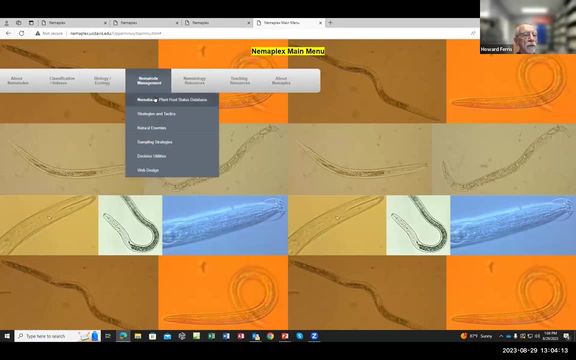 Did you want to share the website again? There we go. That looks good. OK, It's telling me it's closed. OK, so I'm going to NemoBase and I'm trying to think about plant usage. So it's not plant usage, so you go to plant type. 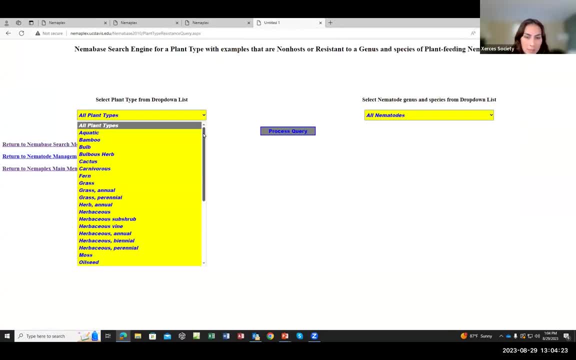 Yeah, it looks like the person who asked this question just actually resubmitted another statement and they said that they found it under a plant type and thank you. So, OK, perennial grass as well. So we're looking at perennial grasses and we're looking at all nematodes. 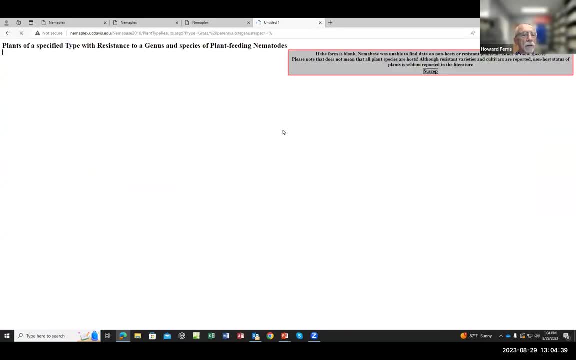 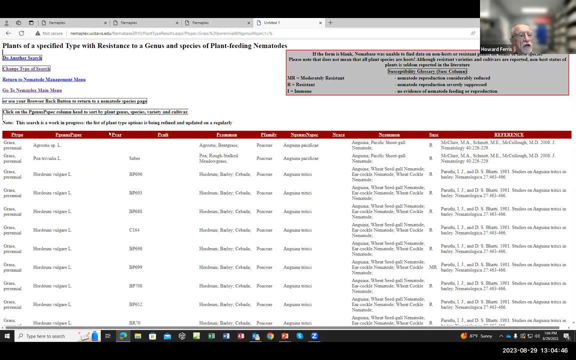 For example: Yeah, So there we go. So now we can say: now I should say that each one of these columns can be, can be sorted. So this is a susceptibility column, I can sort it, and. And so we got moderately resistant. 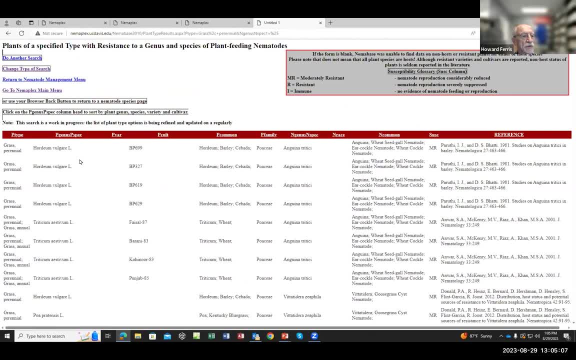 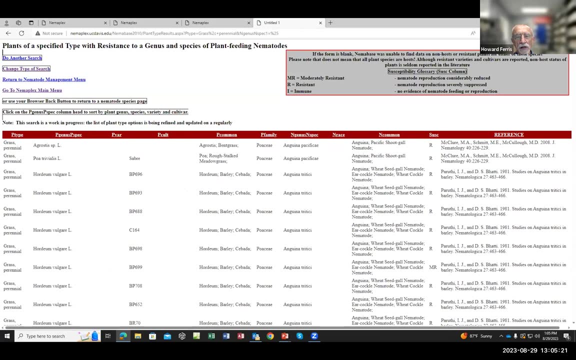 And of course we also need to know what kind of nematode that you're involved here, Right, So I could search by, I could And I've got. I've got. the so important in selecting the perennial grasses is what, what types of nematodes So we've got the Anguina, that is, seed gall nematodes And these are stem and bulb nematodes. I mean leaf gall nematodes as opposed to The Ditalancus. now we're doing with some of the soil nematodes, so we would select also. 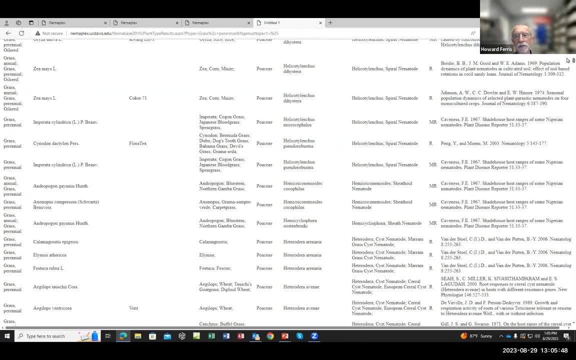 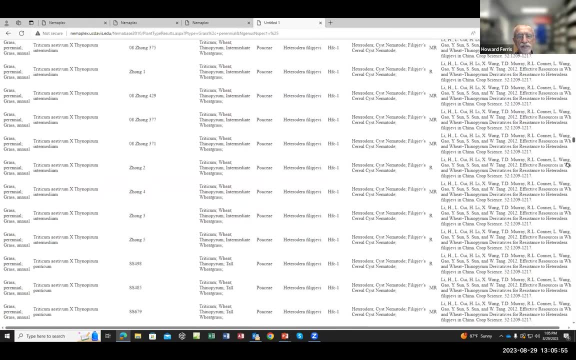 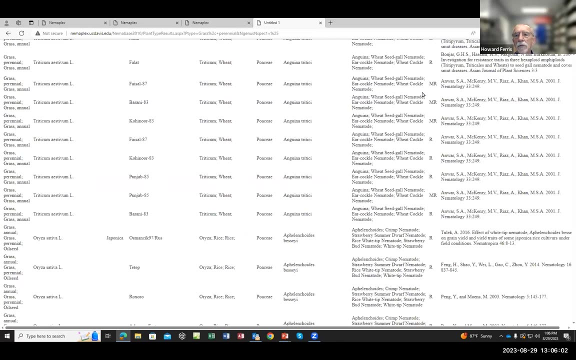 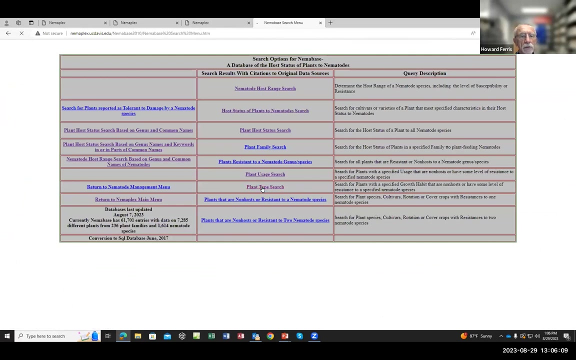 a nematode type that we were interested in, because there are a ton of perennial grasses and we know we want to know who's resistant to what. We went to. Let's see, we go to the top, I go search, And so we want to go back to perennial grasses and we would say we're interested in. 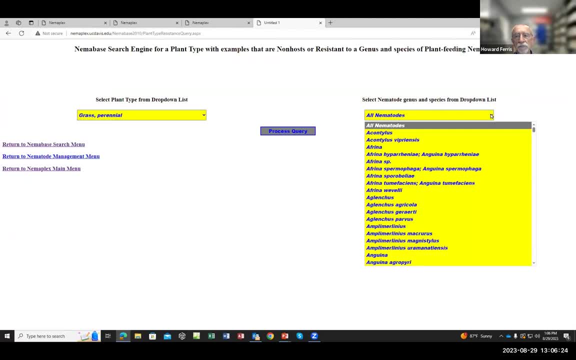 Grass perennial and we would say a specific nematode. Now we're interested in a particular nematode that was in that field And Let's say, I would select- This would be interesting- Globadera, Which is a stich forming nematode. 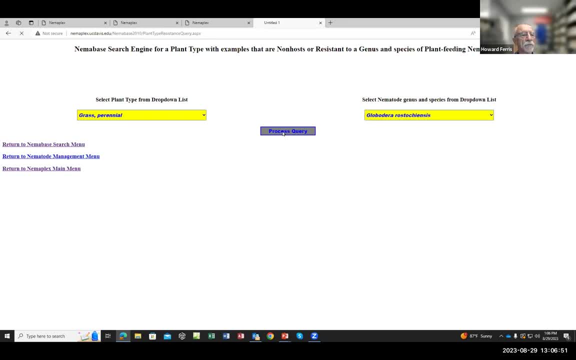 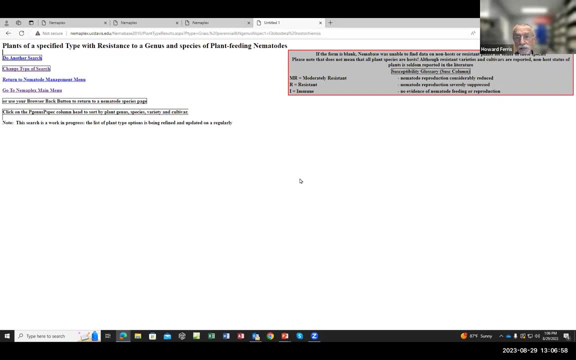 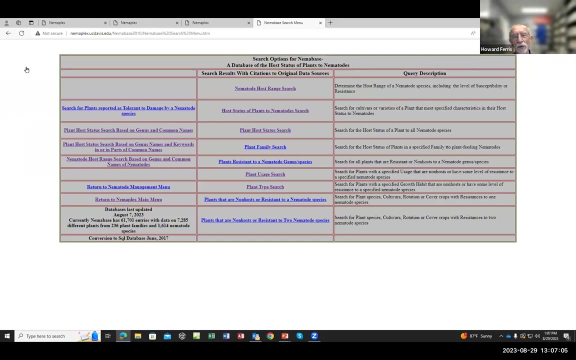 Globadera: rust against the nematode and process query: Interesting, No. Now the fact that it doesn't go any means either I haven't collected the data or nobody did the experiment, you know so. so I'm only reporting what, what. 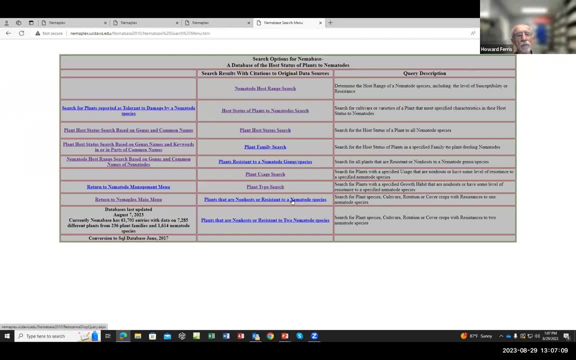 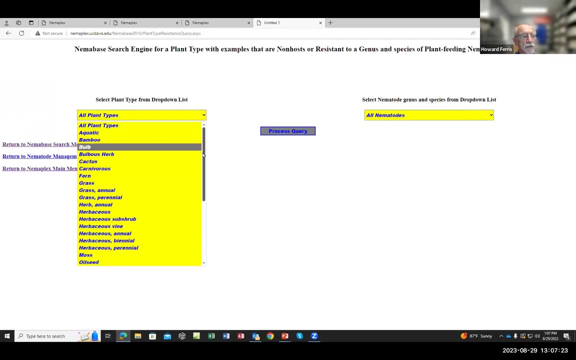 occurs in the literature, and people are more likely to indicate that they that this is a host, then it is a non host. So so it's pretty interesting to to think of the biases that that are That are involved in just the way data are reported or not reported. 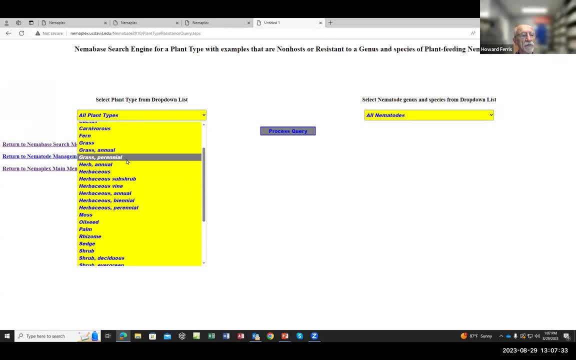 if you don't find the nematode feeding on the root, you don't say anything about it. If you do find this, the nematode feeding on the root, then it's, it's pretty important And you, you would report it. 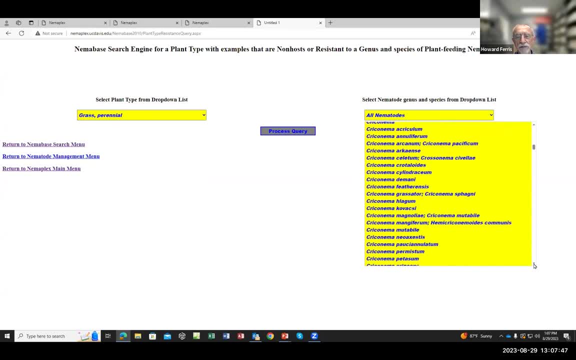 On the other hand, if you're doing a study looking for host plant resistance of plants to nematodes, then then that would become. Let's see. I think in the interest of of time, Dr Farris, several people are saying 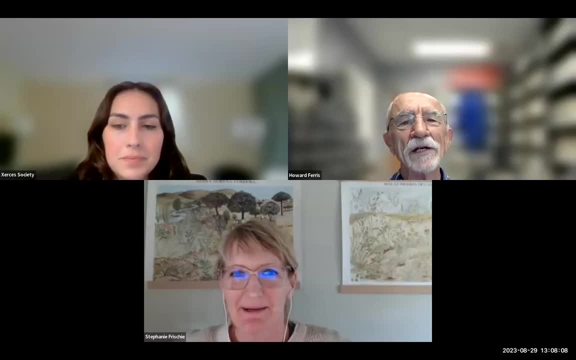 Thank you, And they're having to to jump off here. Well, I understand that I wasn't sort of prepared to do a whole nematode thing, but that was that was good to see some of it there. Well, it's a self-entertainment kind of thing. 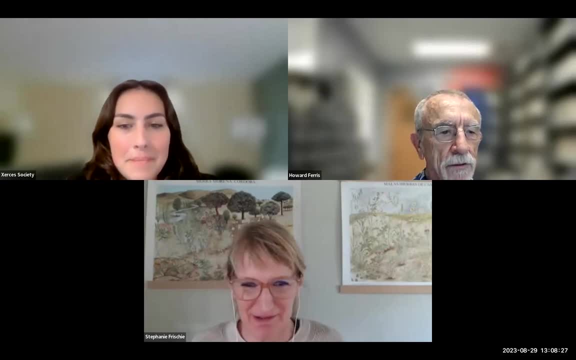 So there's. there's one more question in the Q&A. Let's go ahead and do that, please. Great Yeah. So for biofumigants, does the effect take place after the incorporation of the cover crop into the soil? 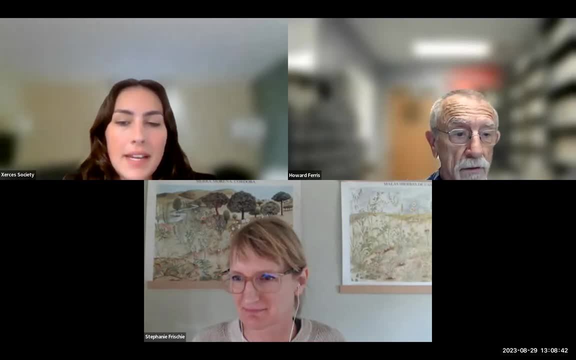 Does the effect occur then? Does the effect take place after incorporation of the cover crop into the soil? Yes, Yes, That's. that's the idea is that the incorporation is kind of breaking up the plant material and the glucosinolate effect is is. comes into impact with myrosinase, which is the enzyme in the leaves, And so it has to be kind of broken up for the enzyme to reach the, the glucosinolate, and that produces the isothiocyanates that kill the nematodes. 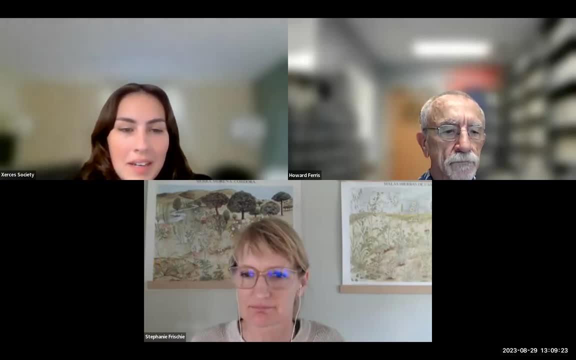 Great, We have a couple other questions coming in. Steph, do we want to stay on for a couple more minutes, or do we? Oh, you're muted. We've got these two here. let's take those and then we'll cut it off. 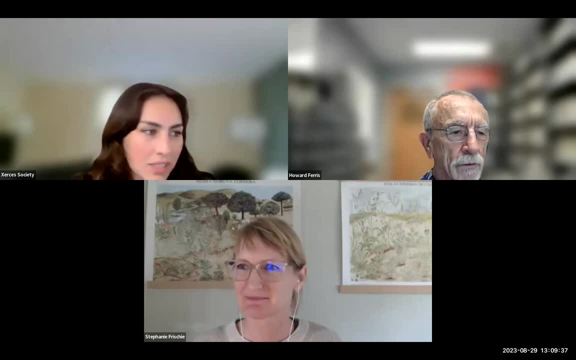 for that. Thank you so much, everyone for the question. Yeah, And of course also, if you do have questions, please feel free to email soils at Xercesorg and we will forward them to Howard and answer them the best. 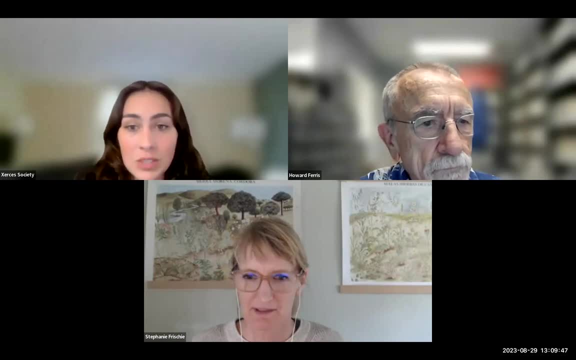 that we can, if you think of anything after this. So now for the last two questions. how can someone get help finding out if a nematode is causing the problem in a crop? So you know, the standard answer to that would be call your local farm adviser. But in California at least, there are a lot of diagnostic labs. not a lot, There are probably a dozen diagnostic labs that provide that kind of service that would would recognize or be able to identify the species of nematodes present and whether or not they were parasitic on the crop that you were growing. If now, with some nematodes there are distinct symptoms, You can see galls on the roots, or cysts attached to the roots or something, And you know, the more cysts, the more galls, the poorer the crop is growing. 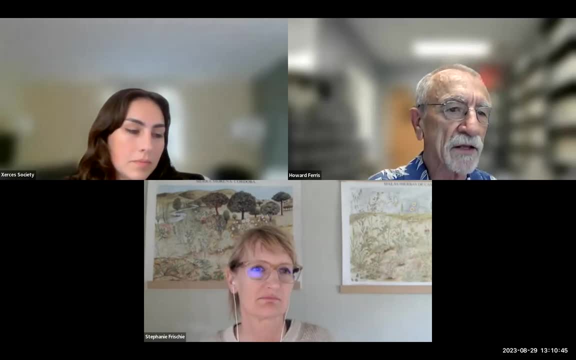 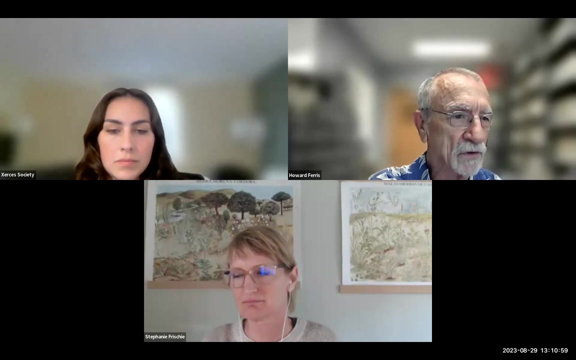 And this is that cause and effect kind of kind of linkage. In other cases there are no obvious symptoms on the plant or no obvious symptoms can be ascribed to a specific organism, other than the plant is not growing as well, or it looks nitrogen deficient or it looks like it wilts in the midday. 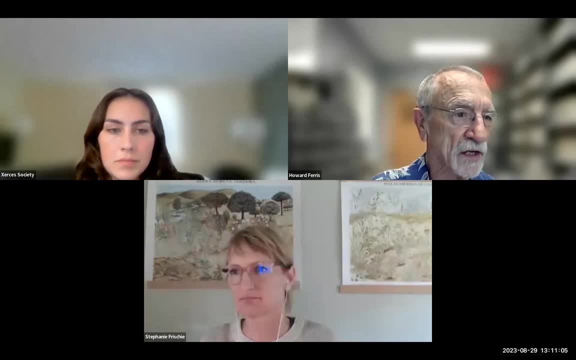 which is usually a pretty good indicator that that something is affecting the roots. And then if you, if you took soil samples and find high populations of plant parasitic nematodes, you'd ascribe them to that, You know, and there's probably are reports.